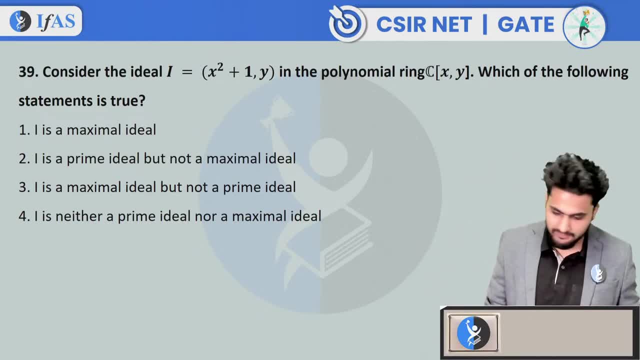 generated by x squared plus 1 and y, The polynomial ring Cxy. which of the following statement is true? Which statement is correct about this ideal Cxy? I will tell you. Take a look, Answer it quickly, what it is, Try it. 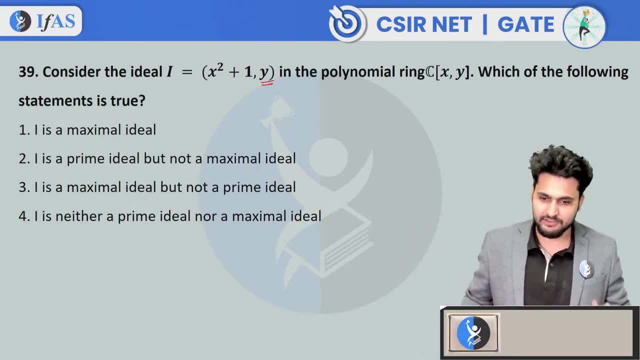 Look at every question. Try it yourself. If it doesn't work, it doesn't matter, We will discuss together. We will discuss the answer together. If it gets solved, it's a good thing. If it doesn't work, it means that there is a question that you don't know. 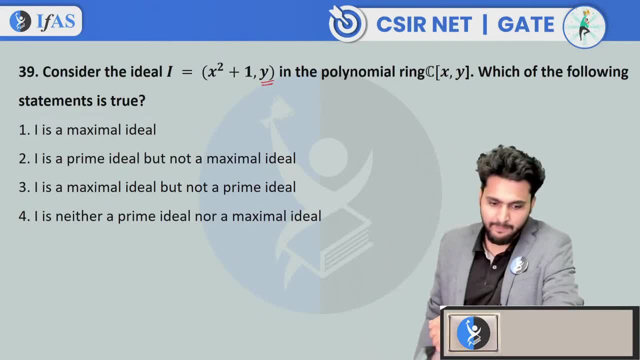 Somewhere you have a problem. When we will discuss, you will get something new, Okay, Good evening Shatna, Good evening everyone. The answer to this question is that the ideal is generated by x squared plus 1 comma y in the polynomial Cxy. 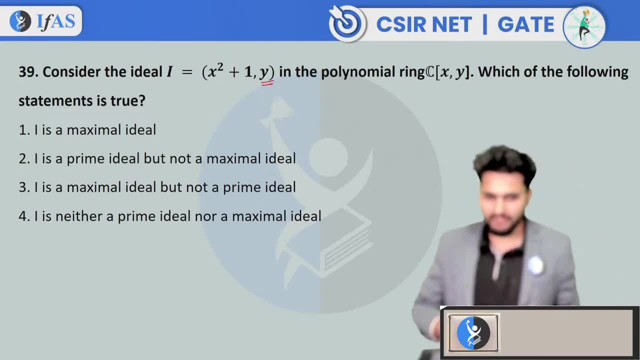 What is the following ideal? Everyone is listening. The answer to the question was: which of the following states is true? Which statement is correct among these? Think and answer with me. Look, Answer it first. If it does not happen, then we will discuss. 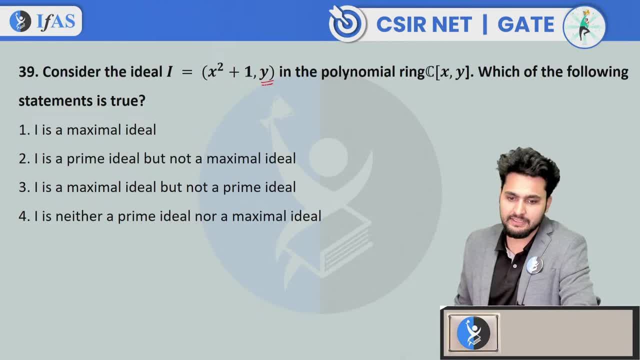 First option is that I is a maximal ideal. Is I a maximal ideal? I is a prime ideal rather than a maximal ideal. Is I a prime but not a maximal ideal? Then I is a maximal ideal but not a prime ideal. Then I is neither a prime one. but it is possible that. 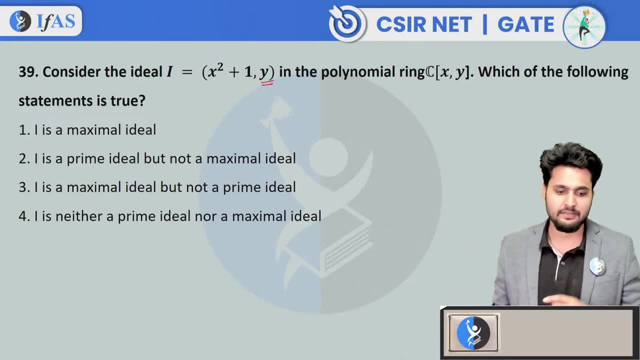 is not so clear. okay, fine, Vishal, thank you so much for your comment. let me take it once. give me one second. let me check if there is any issue. what is the blur for this answer? what is the blur what you all have given? yeah, Yeah, the info looks totally fine. 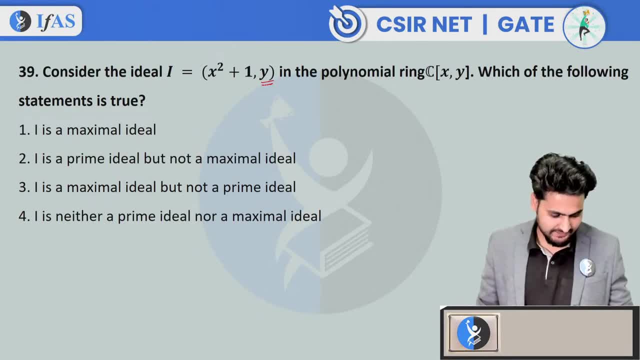 I am still trying to see if there is anything clear. yeah, its on the scan. Oh, my Melissa, you can check it out now. Okay, I hope I have answered some of your questions, So let's move on to the next question. What can be the answer about i? 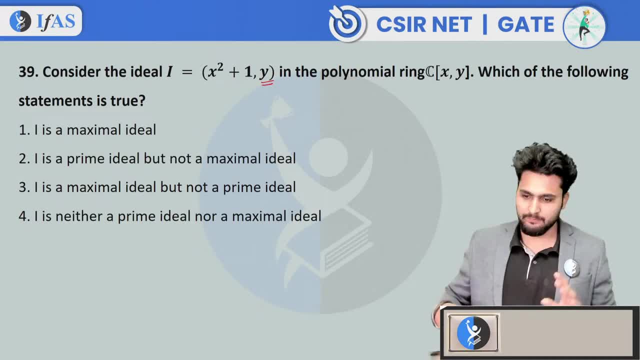 This question is related to the question of the polynomial ring and the question of the ring. If you know some of the key points, then you can answer them very well. For example, you have to see this question First of all. I will write a riddle with whatever I will use. 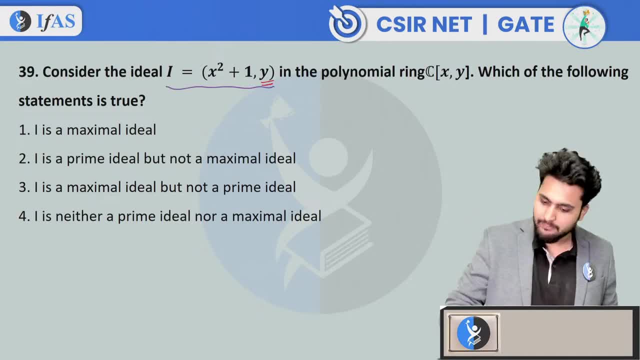 So i equals to ideal generator y. Now we will ask about cxy: Is i the maximal ideal or not? The first riddle is that in a commutative ring with unity i is a maximal ideal and ideal i is a maximal ideal. 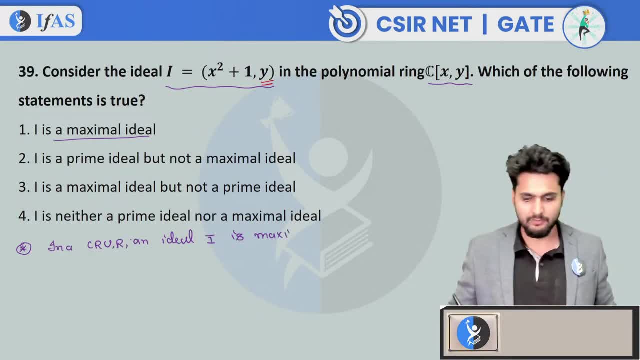 In a CRU, I take CRU as r. In a CRU, I take CRU as r. The commutative ring with unity is r. I will talk about that. i is a maximal ideal. i is a maximal ideal. 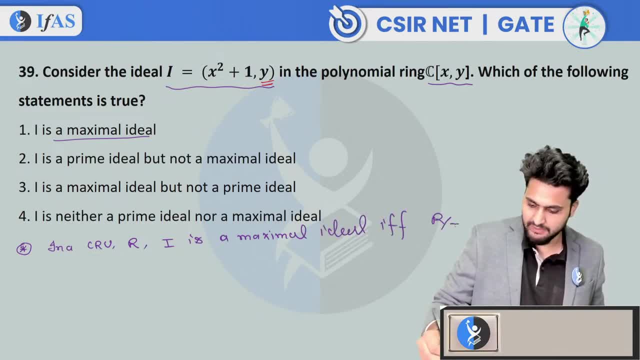 If, and only if, r by i is a field, You can never see directly whether it is a maximal ideal or not. If the quotient ring fails, then we will do the maximal here. What will we do? cx comma y upon ideal generated by x square plus 1 comma y. 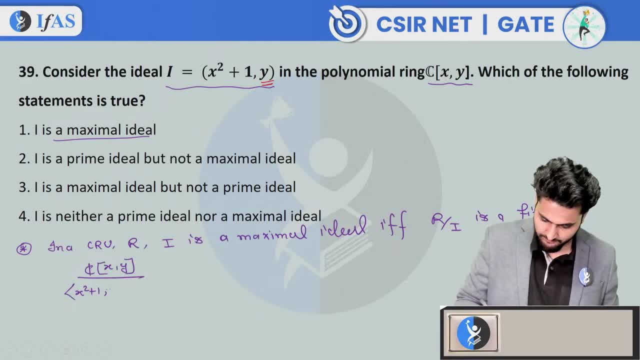 cx comma y upon ideal generated by x square plus 1 comma y. We will see this. Whose isomorphic will it be The y that you see? This y will be in the same place From top to bottom. We will not cancel it. 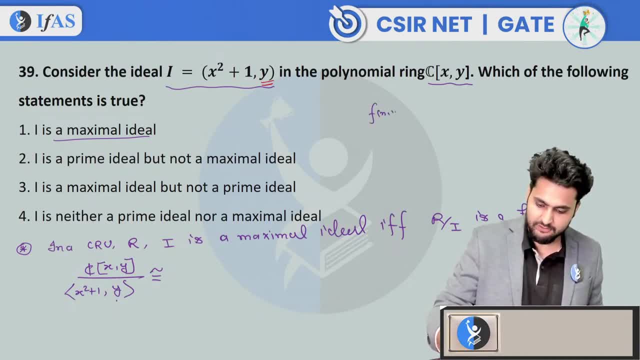 Because if you see any element of this, it looks like this: f of x comma y plus ideal, generated by x square plus 1 comma y. Now, if you see the polynomial f of xy of cxy, If y is coming anywhere in this, then it will be in this: 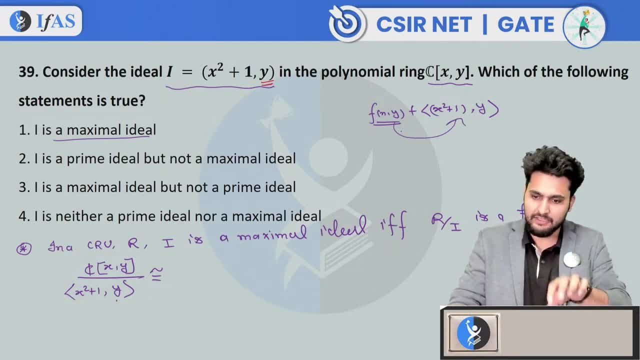 So whatever is left in f of xy. Actually, the polynomial is of cx. So whose isomorphic will it be? cx upon ideal generated by x square plus 1.. Whose isomorphic will it be? What is the name of the algebra? 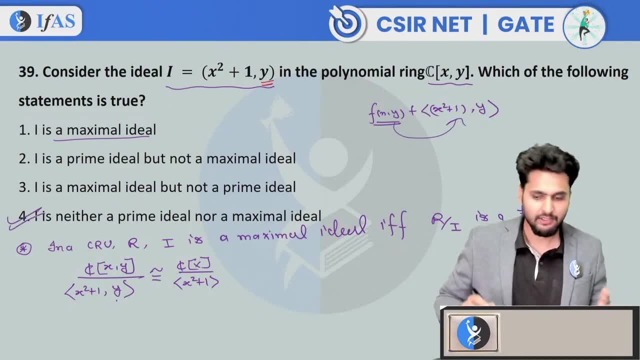 Shanta, you think 4 is correct and you are absolutely correct. 4 is the correct answer for this question. i is neither a prime nor an exponential, And that's it. If you understand whose isomorphic it is, then this is the whole question. 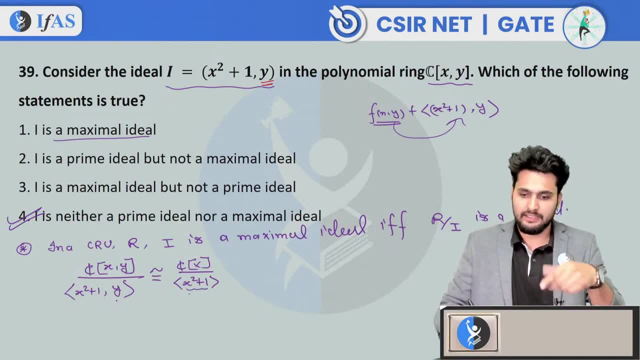 Now, if you see x square plus 1 is reduced to c. So in c All the polynomials are reduced If the degree is greater than 1.. So any degree 2 or greater than that, all the polynomials are reduced. 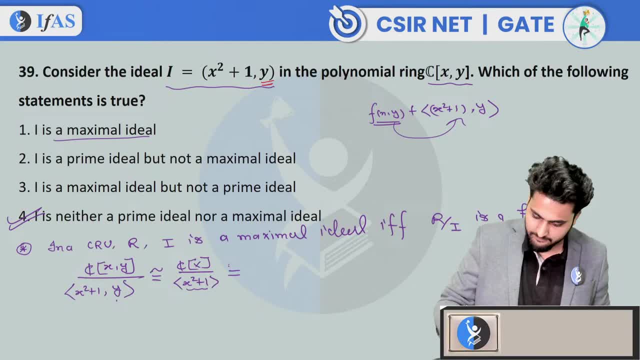 So these two things, Because of the reduction we can write in Chinese. Whose isomorphic is this? First, you write it equally: x plus i into x minus i. These are the factors, Because the factor is not the case. 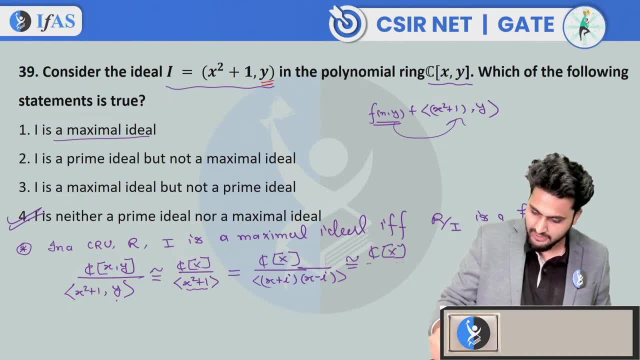 This isomorphic can be different: dx upon ideal generated by x plus i Cross dx upon ideal generated by x. dx upon ideal generated by x minus i. Now, these are the polynomials of degree 1.. Because of these, what will happen? 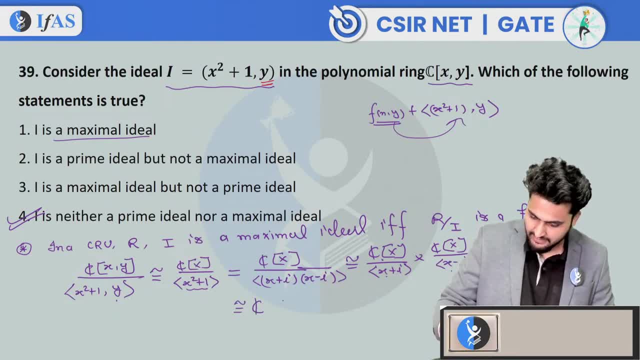 Whose isomorphic is this? Here also c will be left, c cross- Here also c will be left. Whose isomorphic is this? c cross, c, D is the correct answer. Okay, Whose isomorphic is this? 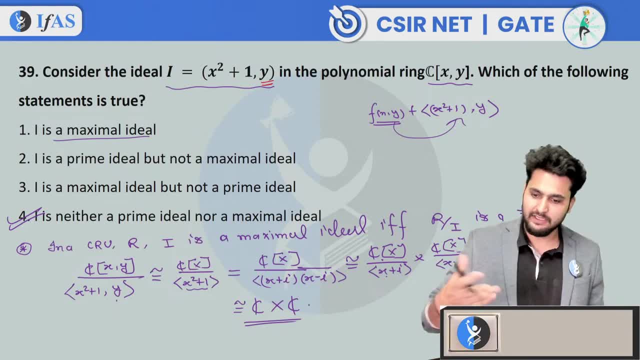 c, cross c, And if you see, whose isomorphic is this, Whose isomorphic is this? We are done. This is not an integral domain. Not an integral domain. This is not an integral domain either. It has zero devices. 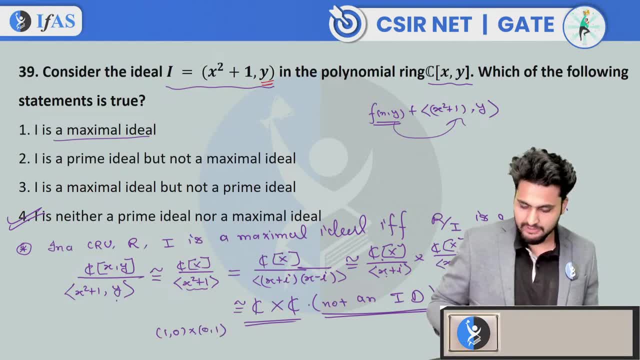 We will consider 1 comma 0.. 0 comma 1.. This is a non-zero element, But you get 0, 0 to product it, So this is not an integral domain either. If this is not an integral domain, then there is no field either. 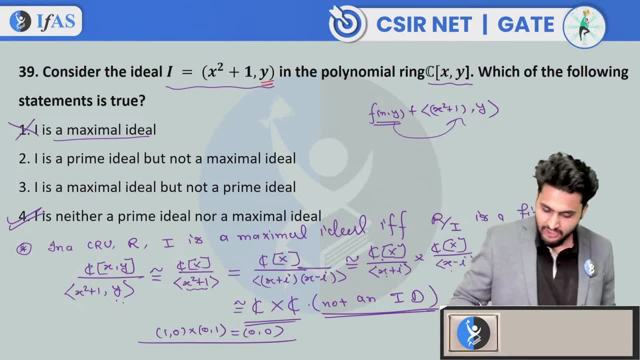 There is no field, So it cannot be a maximal ideal And it is not an integral domain, So it cannot be a prime. So you can click on the reason if you want. It is cancelled. You can see here. 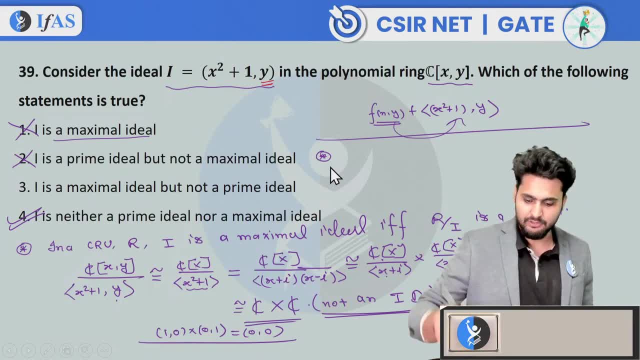 In a CRU. I have understood that I am taking a CRU, So what do you see? i is a prime ideal. i is a prime ideal, Prime ideal, If, and only if, r by i is an integral domain, Integral domain. 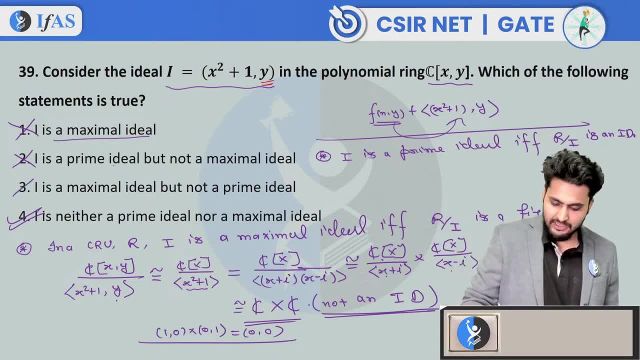 This is the result, Right. Since it is not an integral domain, then it will not be a prime. i is a maximal and prime. Both of these will be wrong. Fourth option: Since it is not an integral domain, then the ideal i is neither a prime nor a maximal. 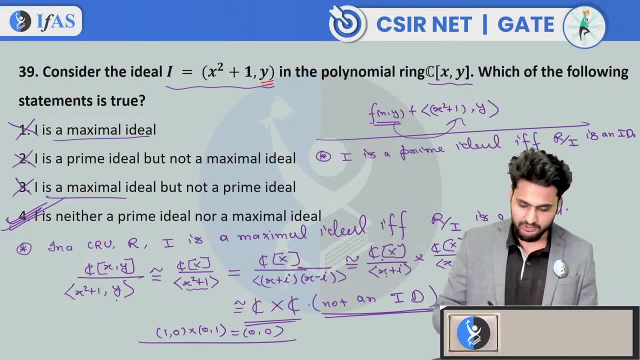 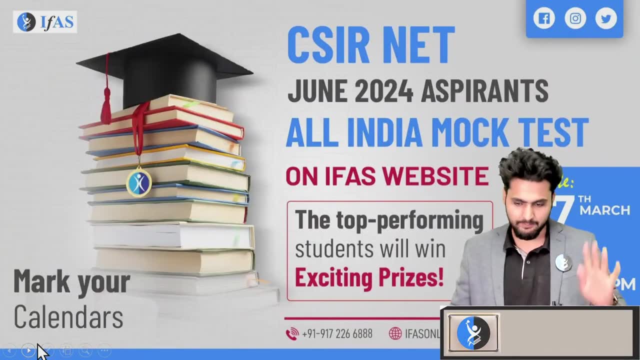 ideal: See x comma y, is there? Okay, So 4 is the only correct option for this. If anyone has any problem or confusion, don't worry, It is not an integral domain. Okay, Next question. Before looking at the next question: 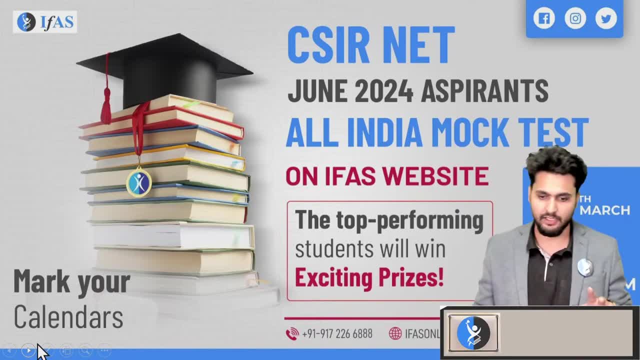 If you are preparing for CSI and NET's upcoming exams, then you have to organize a free mock test for all of you. What do you have to do? You have to give. It is absolutely free. Along with that, if you get a good rank, then what can you do? 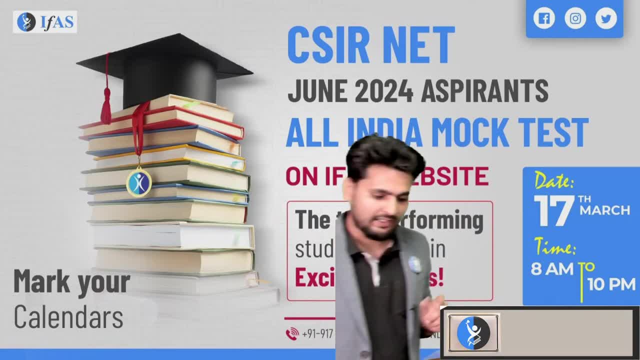 Exciting prizes are also available for you, So you can win them. And when do you have to give? 17th of March, It is absolutely free. You have to go to the website of IFH and give this 17th of March. 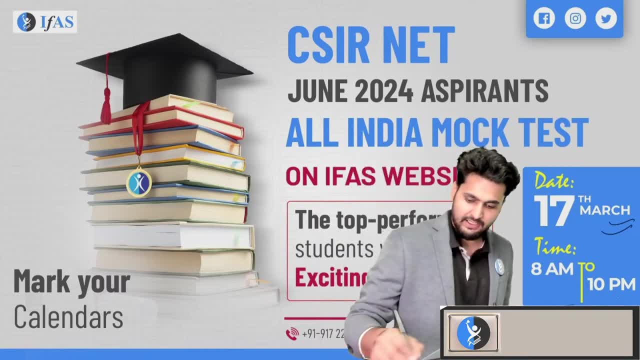 From 8 am to 10 pm. Between 10 am and 10 pm You have to give Okay If you are preparing, then nothing will happen. Your question will be practiced. So you all have to give once Okay. 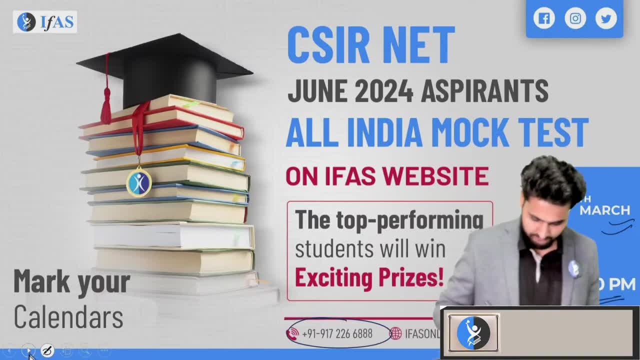 If you have any problem, then you can get a call on this number. Okay, Let's see the next question. Let R and equals 2.. This is a very good question. This is a previous question. I will tell you all, to try. 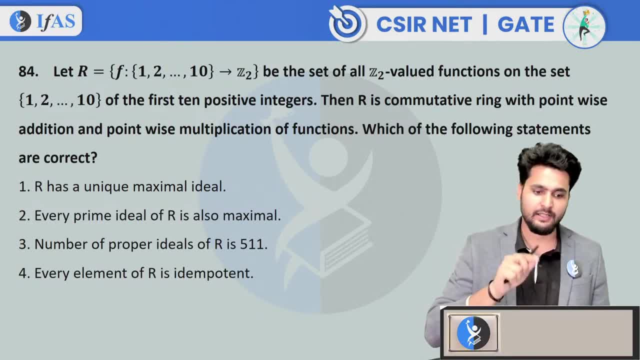 If it doesn't work, then don't believe. If I will explain to you, then I guarantee you that you will understand. Okay, So look at this and then answer it. Read it yourself and then answer it. It is a very good question. 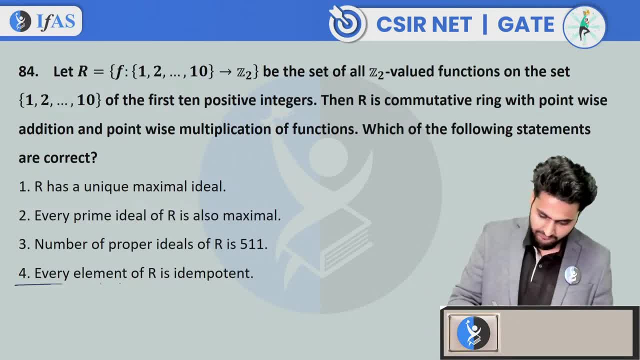 It is a previous question. It is a very good question. It is a very good question. It is a very good question. Look, attaboy children Read the question and then answer it. This is a very good question. When you will understand this, then you will believe. 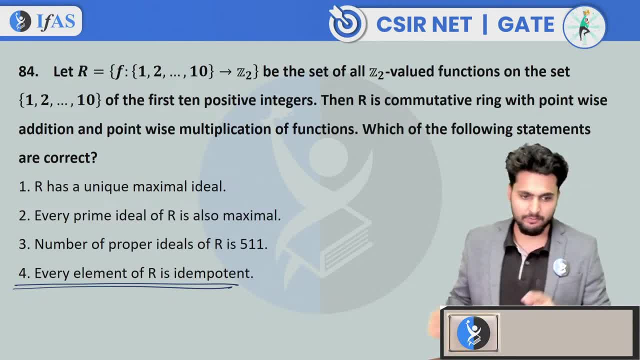 This is actually a very good question. Write this because this is the collection of all the holidays. This questions is in Internationalé. Okay, functions from this set. This is a set with 10 elements and z2 is the map. All the functions. 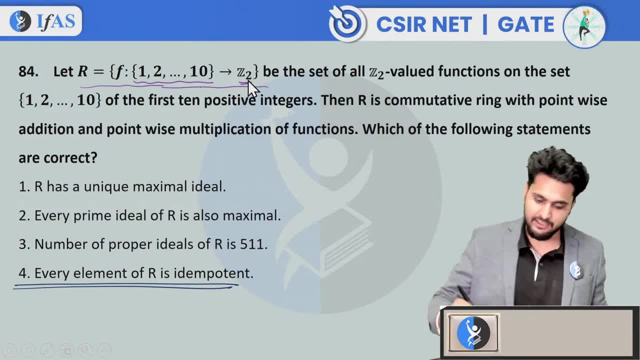 from this set. all the functions that can be defined on z2 are called r. This is a set of all z2 valued functions on the set 1 to 10.. That is what I told you Of the first 10 positive integers set. all the functions that can be defined on z2 are called r. Then, 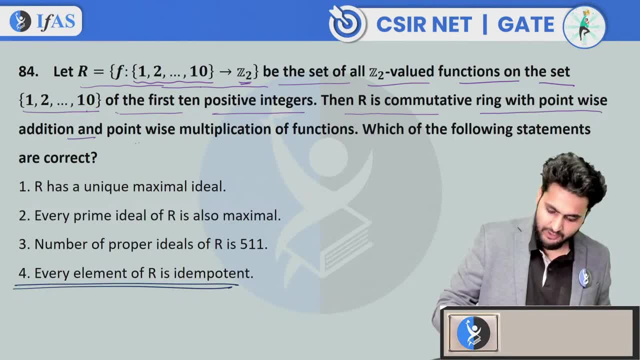 r is a commutative ring with the pointwise addition. In respect of pointwise multiplication, this ring will also be made: Pointwise addition means f plus g at x will be defined as f of x and g of x. Multiplication. g at x is defined as f of x into g of x. With respect to this, 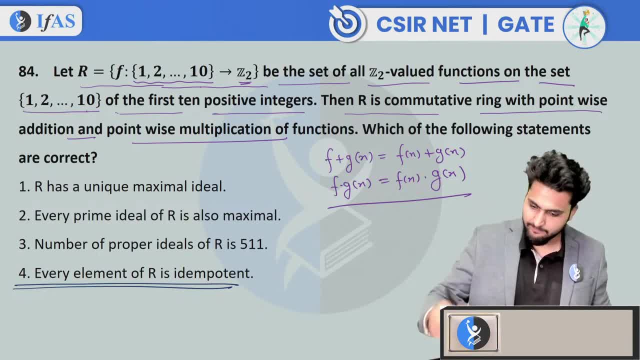 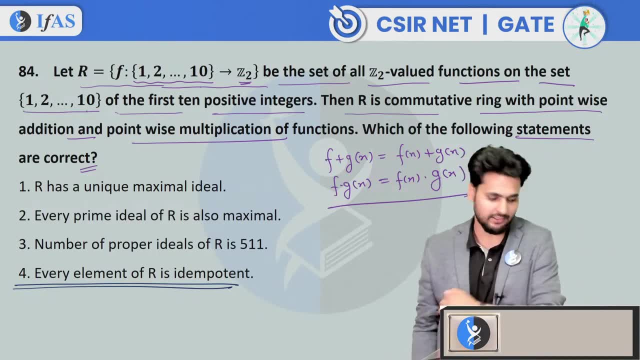 addition and multiplication of this, a commutative ring will be made. Then what will happen? Which of the following statements are correct? Which of these statements are correct? Think about it. What do you think? The previous question is yes or no. 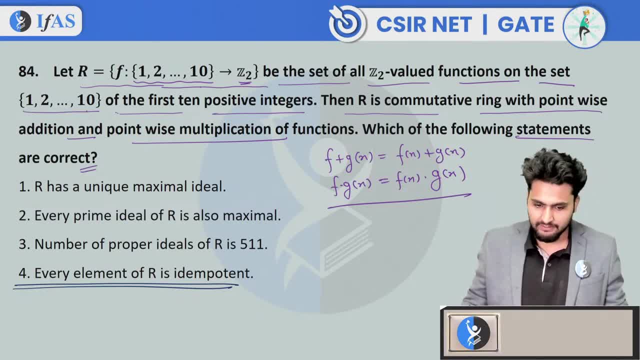 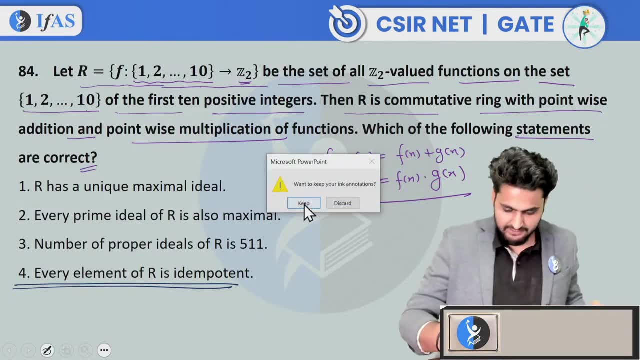 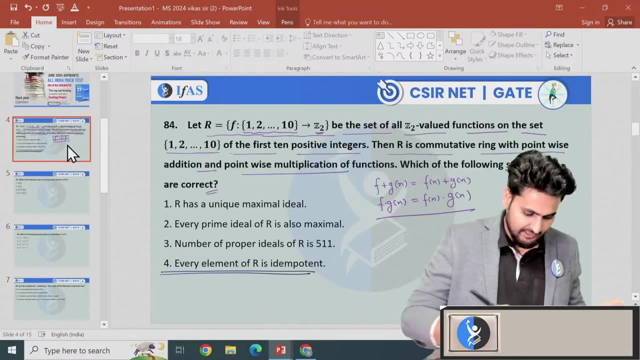 Look at this. If someone has any understanding, he will immediately answer and tell me. Let me see how you think I will do one thing: I will add my base and I will explain to you how we solve this. So if you look at this ring, first of all I will ask you how many. 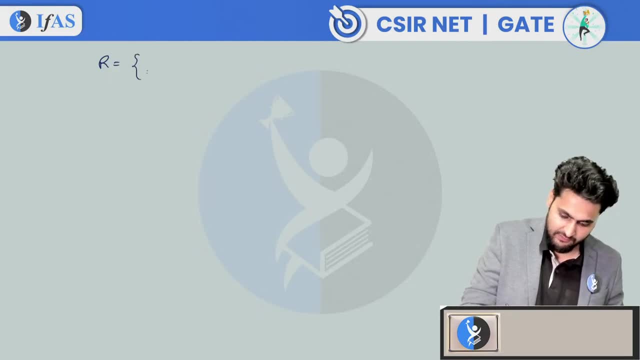 total elements are there. in this r is the collection of all the functions which can be defined, which are defined from 1 to 10.. 1,, 2,, 3, 4, 5, 6,, 7,, 8,, 9, 10.. All the functions can be defined in z2,. 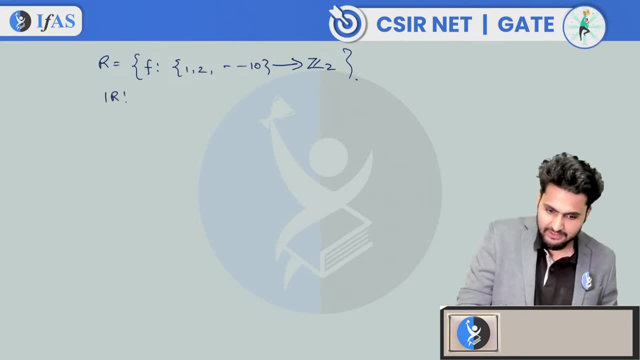 all of them are collected. So what is the cardinality of r? If you look at r, then our total function is defined here. If you know the cardinality of a, then you can find out the cardinality of b. How many functions can we define on a and b? 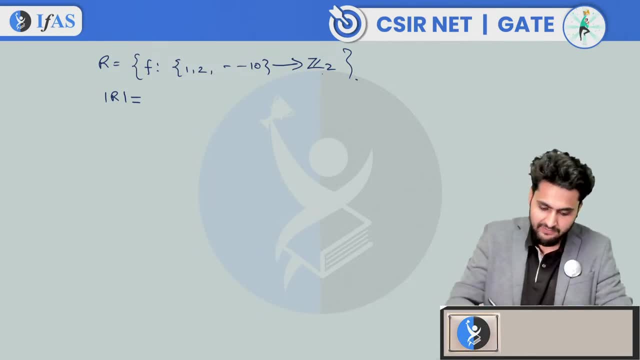 Which is nothing but the cardinality of b. So the cardinality of b is 2 here. What is the cardinality of 2?? 2 to the power. What is the cardinality of this? 10.. The cardinality of b is 2 to the power, 10. It is arrived by this. 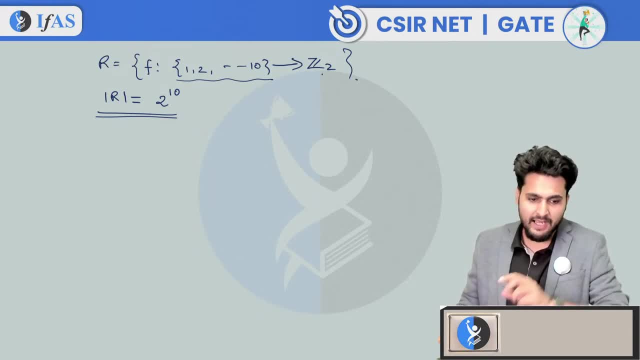 So here it seems a little ideal. that whose isomorphism can it be? Let me tell you: this is isomorphism 2 times r is isomorphism z2, cross, z2, x, z2 10 times. whose isomorphism is this? Ours is okay, 2 to the power 10? Correct? 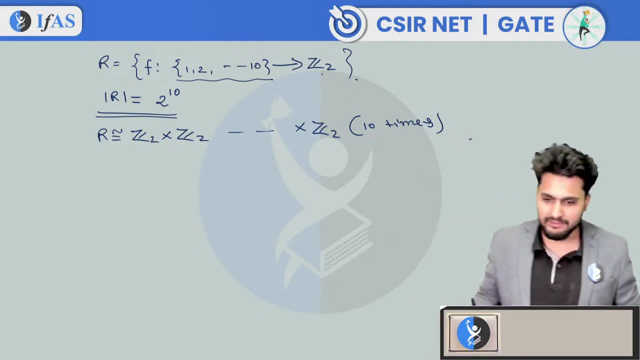 There is 2 to the power 10 element. I will not let you verify this if I say now I will totally verify. If 2 to the power 10 is element and 2 is a 2, that means Hopefully I will. 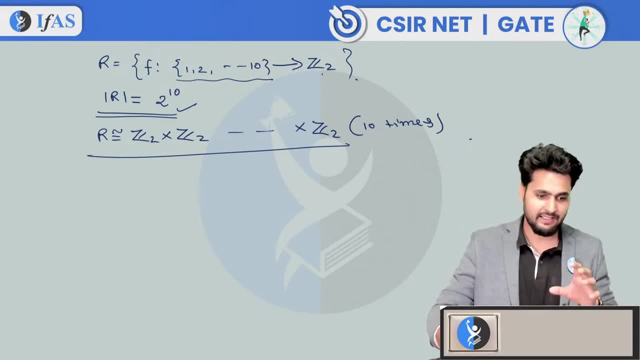 So this is isomorphic of this, but this will only come to you if you have done such a question once or if you have an idea that such a function, collection ring, is isomorphic of cross product of Z2, right, So let's verify this that, yes, this is really isomorphic. 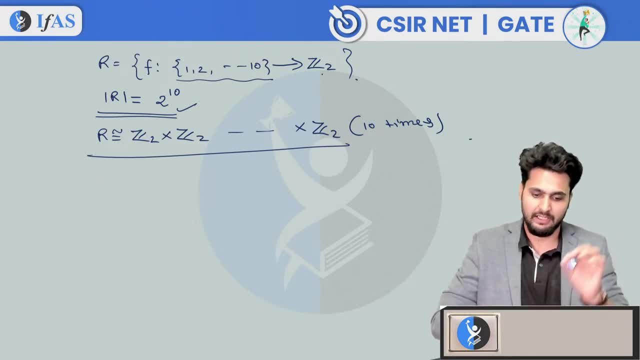 For isomorphic. if we have to divide two rings by isomorphic, then what should we do? Isomorphism can be defined, so let's define an isomorphism phi from R to Z2, cross, Z2, cross, Z2, cross, Z2: 10 times. 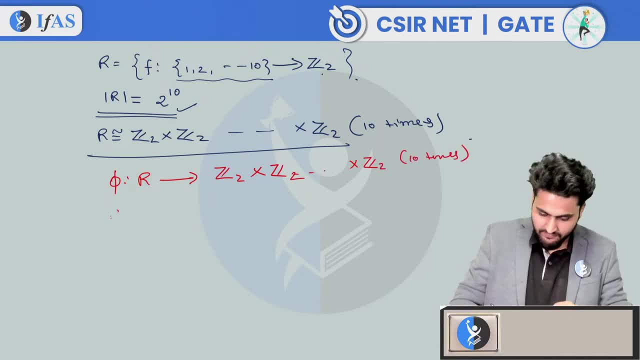 Let me tell you a map. If I have considered any function f, then Z2 cross Z2 10 times will come here. So any of you who are watching, any of you want to know what can be a map. I have considered this function f from here. 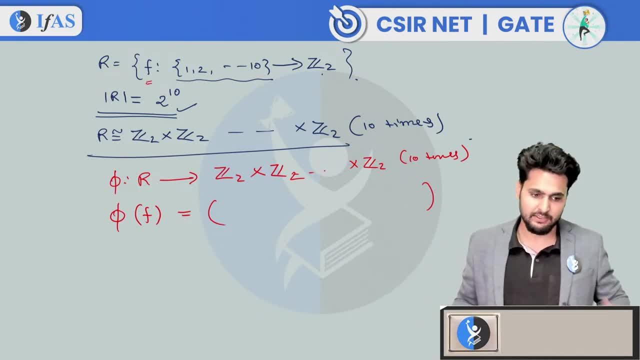 I will make this function a map on the element of Z2 cross Z2.. What can be a function? What can be a guess? What can be a natural guess? What can I define? Anybody? Z2 cross Z2.. We need an element of Z2 cross Z2 which is corresponding to f. 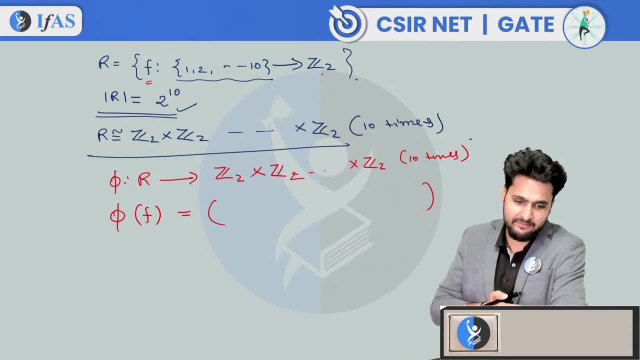 f is the corresponding element. We have to keep f in the image because we have to map f. What can be done? Let me tell you. This is the map We can define: f1 comma, f2 comma, f3, up to f10.. 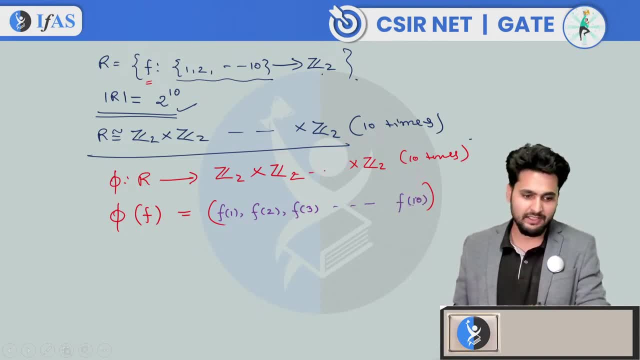 What will we do with this map? We will define it, This function that you are seeing, the map phi that you are seeing. this is an isomorphism. We can verify this. Verify that phi is an isomorphism. Phi is an isomorphism. 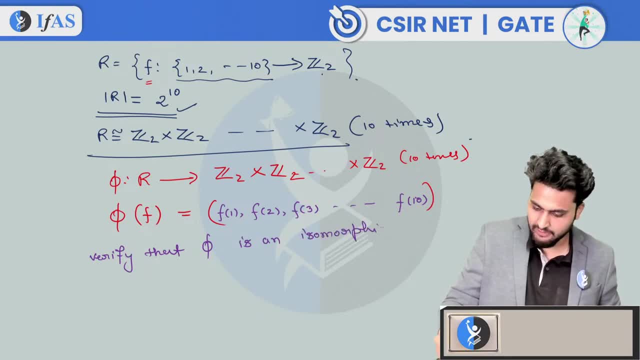 Don't worry, we will verify it. So don't worry, we will just listen to it. We will verify it. This is an isomorphism. What should be done for an isomorphism? What is a ring isomorphism? 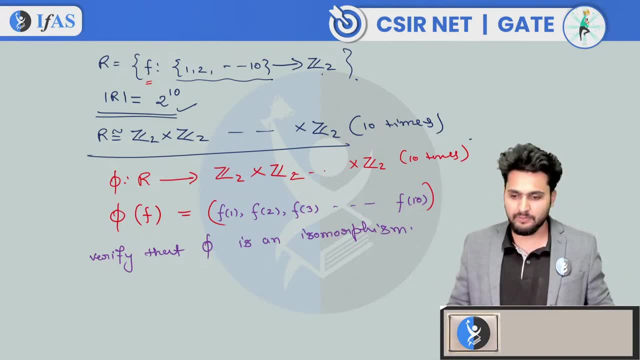 In the case of a ring, if there is a map, then what will be the isomorphism? When it is a binary map, the first thing is that it is 1, 1, 1, 2.. And along with that, it preserves operations addition and multiplication. 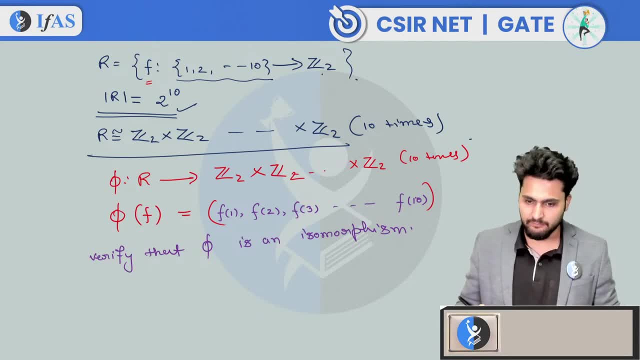 Now we will see that. how is it? It is a bijective. It is 1, 1 and 1, 2.. If I don't verify 1, 1,, then 1, 2, because the operations of the sets on both sides are the same. 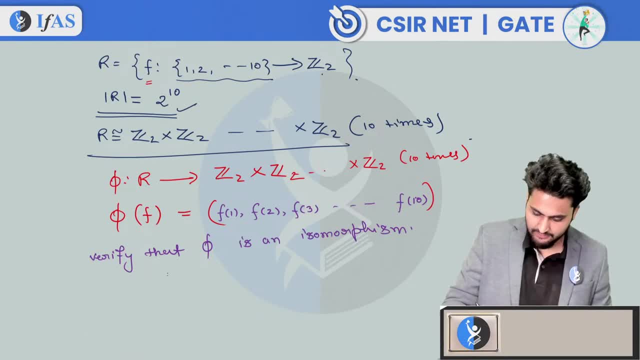 So I will verify 1, 1.. To verify 1, 1, if I show that the kernel of phi. this is our claim. Our claim is that if there is a kernel of phi, then there is only 0 in it. 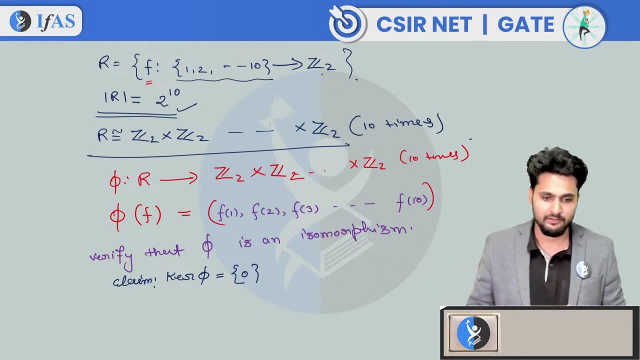 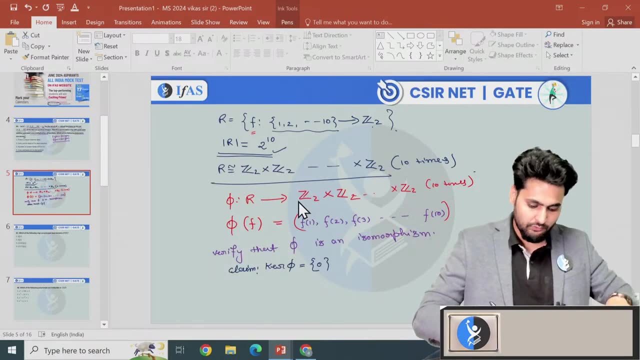 There is 0 function in it and nothing else 0.. We can prove it, We can show this. How can we show this? If I consider a function, it is a kernel. So I will show this. So I will show that this can only be a 0 function. 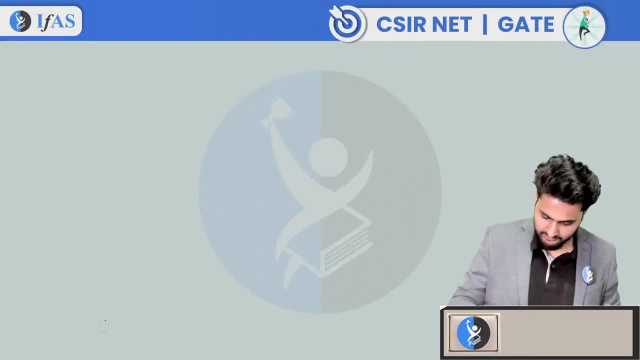 One second, Let's see. Let me consider: Let f belongs to kernel phi. Kernel phi is minimal. What does this mean If phi of f equals to 0 and 0 element is of z2 and z2.. So z2 and z2 are 0 elements. 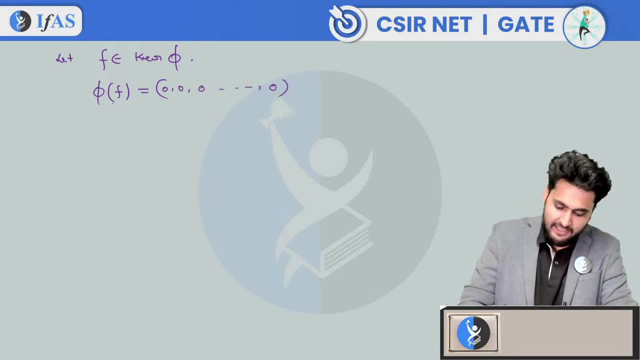 0, 0, 0, 0, 0, 0.. Okay, Phi of f equals to this. And where will phi of f map? We know where phi of f will map: F1 comma, F2 comma, F3. 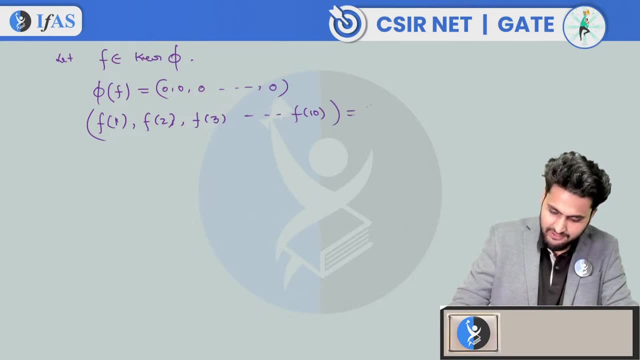 And what should be: f 2 comma, F3?. F5 comma, F6 comma, F7.. F2 comma, F7.. f2 comma, F9 comma, f9 comma, f10.. Right, And how do I use this? 0, 0,, 0, 0. 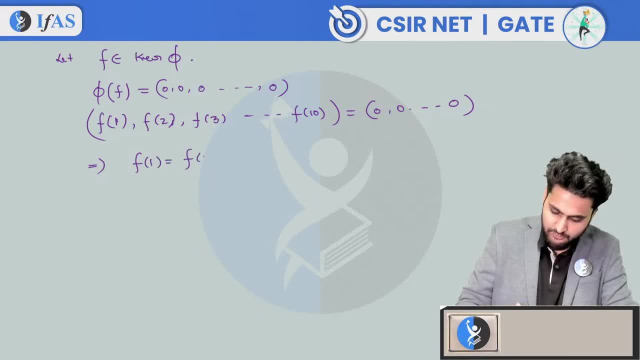 If you make a guess here, What has happened? H1 is a 0, h2 is a 0. They all are equal to 0 and f10 is equal to 0. This is how I am focused on 0. 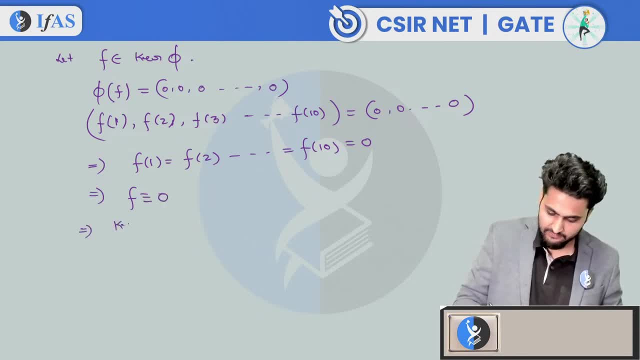 What has happened if the function of 0 is an equal to 0? We canüber apply this to zero function. f is a 0 function. You canиз the fact that kernel phi is trivial. Kernel phi is trivial. Kernel phi of f remains trivial. 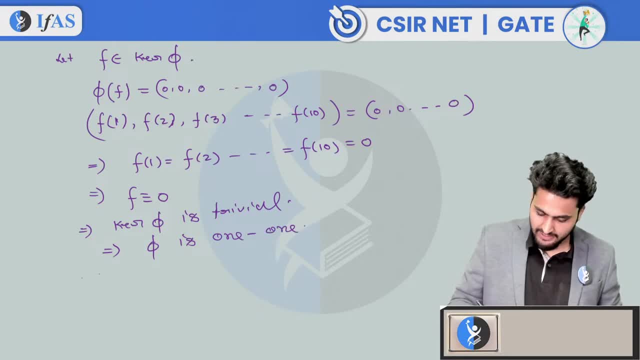 phi is 1,1 and also you can prove that phi is, which implies that phi is onto. also phi is onto. ok, so phi is 1,1 and onto. both have the same identity. so we have everything: 1,1 is onto and 1,1 is objective. now what you have to do is 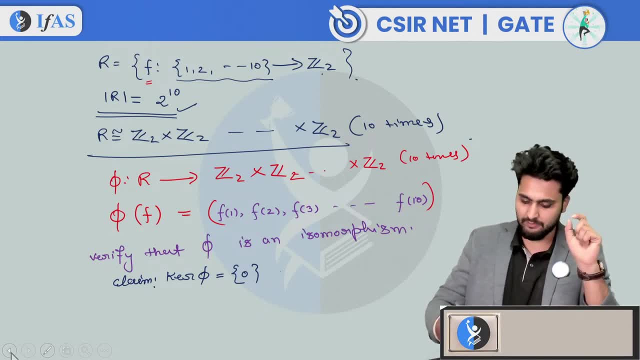 phi also preserves the operation, so it preserves the addition as well as the multiplication. if I take out phi as f plus g, this is equal to phi. here plus phi is also very interesting. I am really interested in this, so I will do it once. 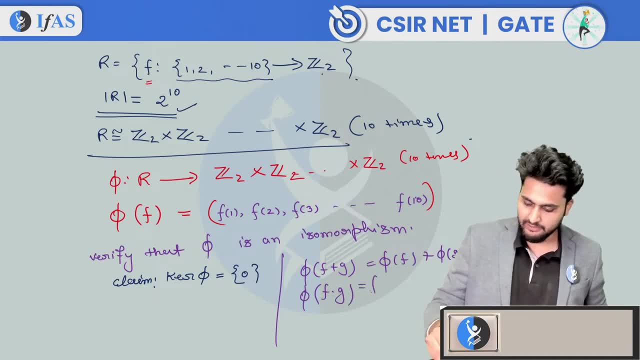 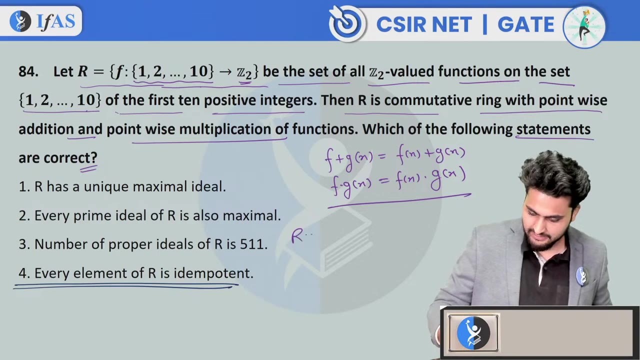 so phi of f into g, this is equal to phi of f. it is very simple. if you have understood this, you can do this as well. all the things are there. so what will happen? it will become isomorphic means. our ring has become isomorphic. r is isomorphic to z2 of r, z2 is given. 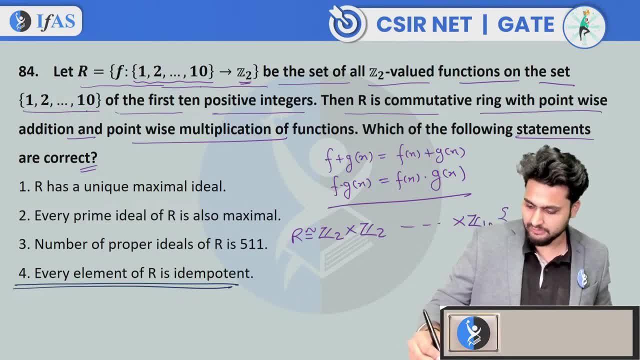 whose isomorphic is it? so this is very easy question. this is 10 times. all the other things are there. whatever you have been asked, you can get it out easily. so what is the next option? good evening to you, good evening to everyone. 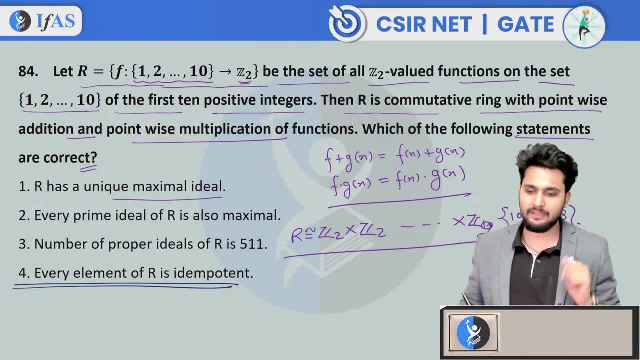 so r is the unique maximal ideal. does r have unique maximal ideal? why? because it has a lot of maximal ideals. how will you tell the maximal ideal from here? you take the maximal ideal. the rest of the ring is the same initially. good evening, good evening. good evening ok. 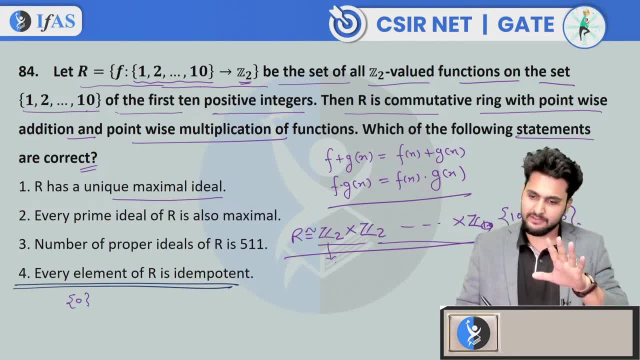 from here you take the maximal ideal: z2 is a field, so it has k equals z. this is the maximal ideal. so we can consider 0 cross z2, cross z2, cross z2: one is the maximal ideal. this is the maximal ideal. 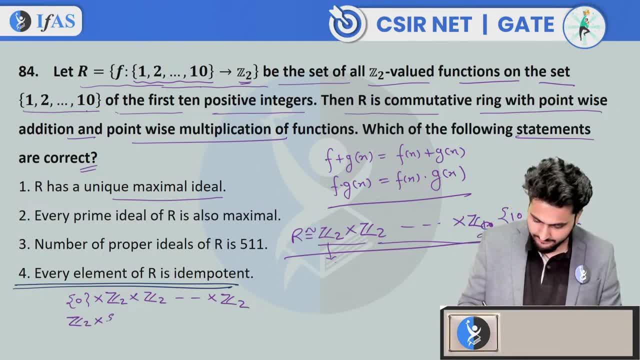 so what will I do now? here I will take z2, here I took the maximal ideal: cross z2, cross z2, cross z2, so many maximal ideals can be made. two is the same, so this is wrong. r has unique maximal ideal. this is not correct. 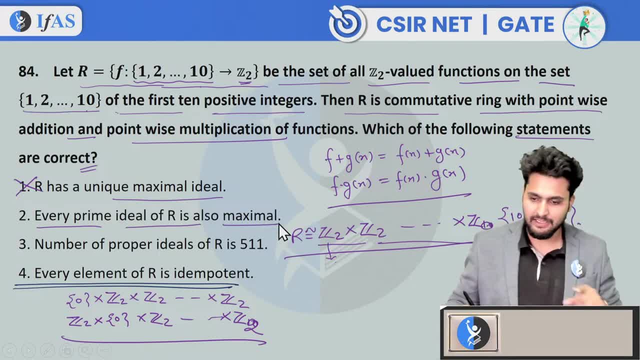 now let's look at this: every prime ideal of r is also maximal. if I consider the prime ideal, then it will be maximal for this, even if you didn't know this, then also you can do this. how can we do this? because here it is said that commutative ring is CRU. 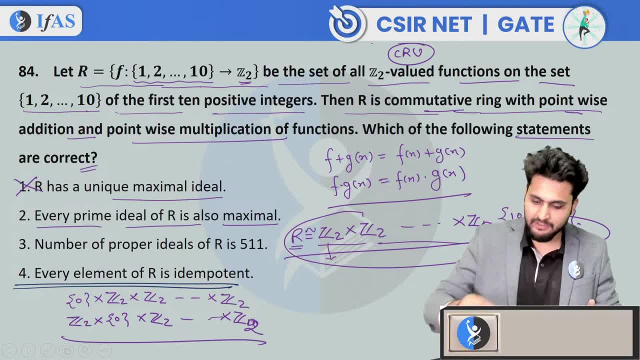 commutative ring with unity along with that, it is finite. you can tell like this: we understood this from here just now. you told that how much is the marginal of r? it is 2 to the power 10. so it will be like this: it is finite, CRU. 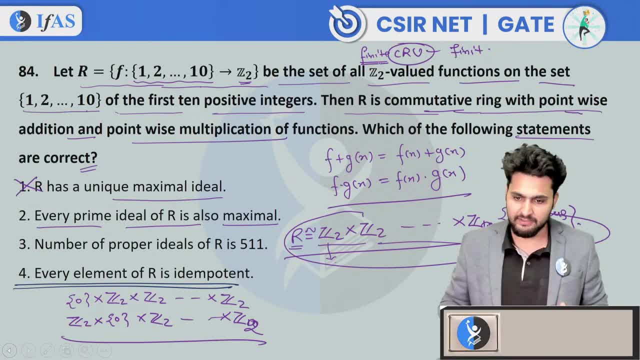 finite CRU means prime ideal is maximal. you know that every prime ideal of r is a maximal ideal, since it is a finite CRU commutative ring with Q. is that ok? we are not true. so why do you think it is not true? 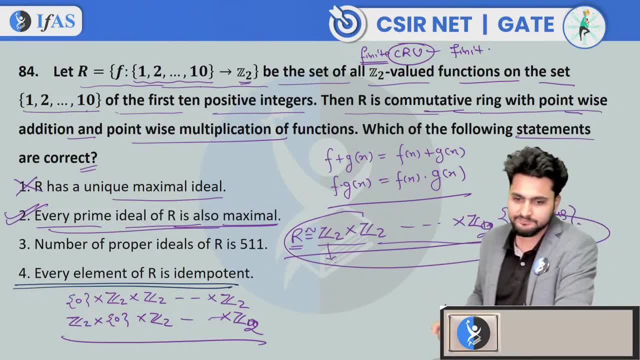 why do you think it is not true? it also has unity. what will be the unity? it is an identity element which will fix every element. we can't fix it here, but we will have it ok, fine. so what do you think? 2 is correct. actually, every prime ideal of r is a maximal. 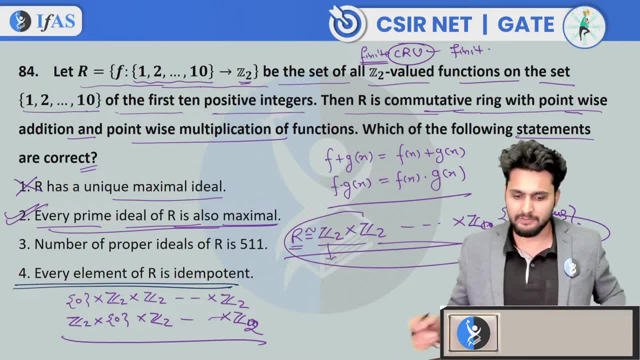 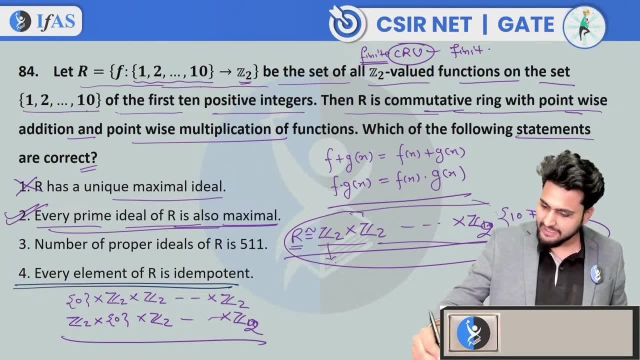 it is a finite commutative ring with unity. so this will be, if you understand, finite CRU from here, then it is correct. if you see here, then you can also say: this is a commutative ring with unity and 5 is finite CRU. 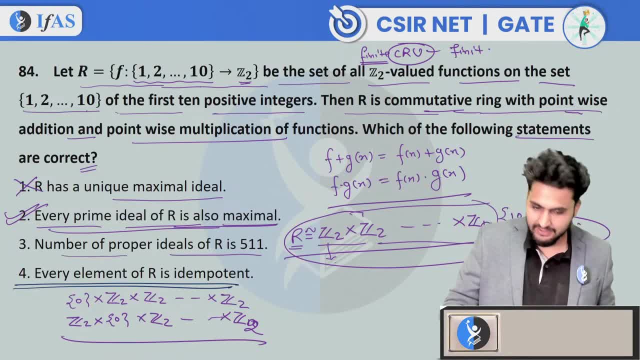 so this is correct. next, number of proper ideals of r is 5, 1, 1. let me tell you: C is not correct. why? because number of ideals of r is nothing but the number of ideals of this ring: z2 cross, z2 cross, z2 cross. 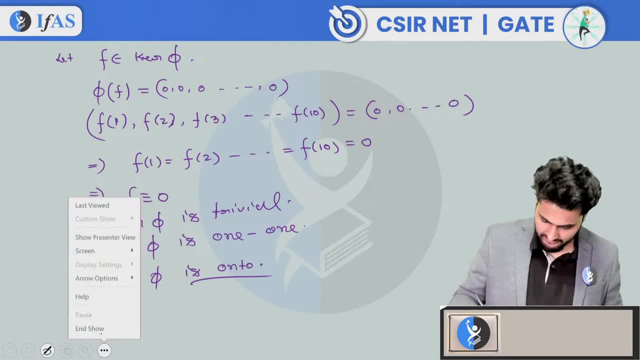 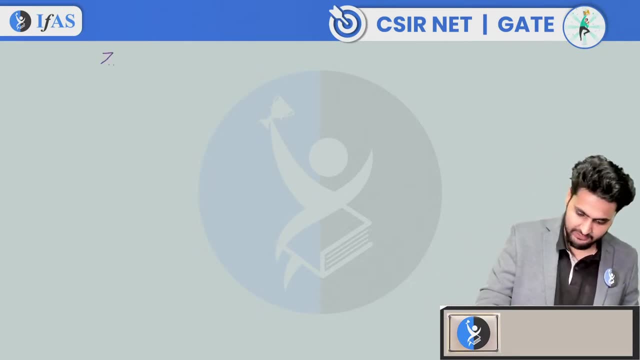 so, in this way, what is the ring we have? z2 cross, z2 cross, z2 cross. let's talk about this. how many ideals does it have? proper ideals: z2 cross, z2 cross. this is also a very good option: z2 cross, z2 cross, z2 cross. 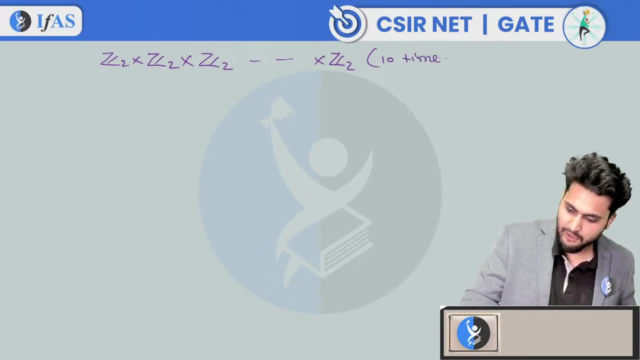 how many times did we take this? 10 times. does it have proper ideals? how many times do we have to think that it has proper ideals? if I ask you how many total ideals it has, its total ideals include 2. it is a drying region, so it only has 2 idols. 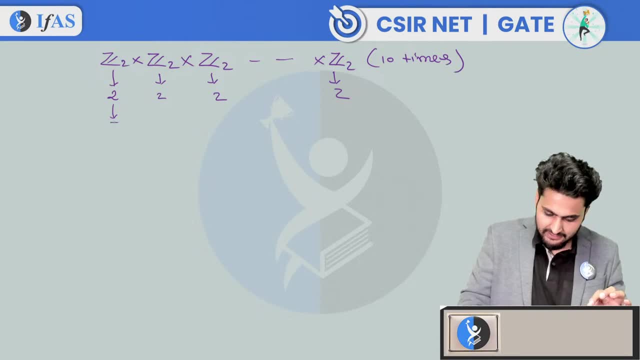 so it only has 2 ideals and if I consider any of these ideals from here, let me consider: from here, i1, and from here i2, i3, from next point, and from here let me take i10. so when you cross it, i1 cross our i10. 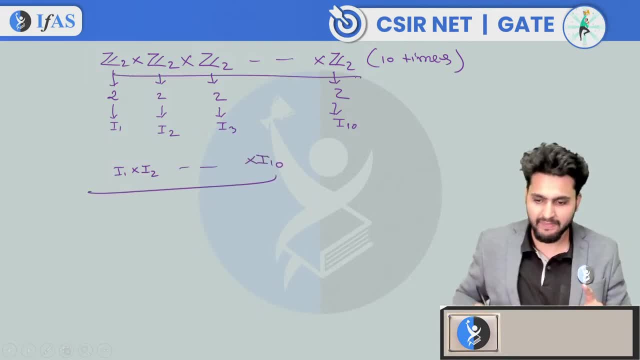 this will be the ideal of w. So if you think, how many choices does i1 have? 2. How many choices does i2 have 2. How many choices does i3 have? All of them have 2 choices. So how many total choices do you have? 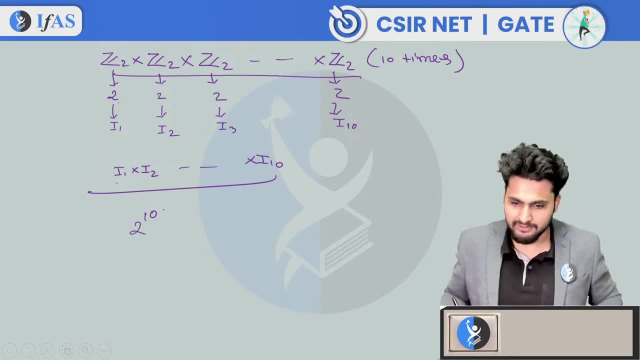 2 to the power 10.. How many choices do you have? 2 to the power 10.. But keep one thing in mind: we talked about a proper ideal. If I take z2 as an ideal from here instead of i1,, 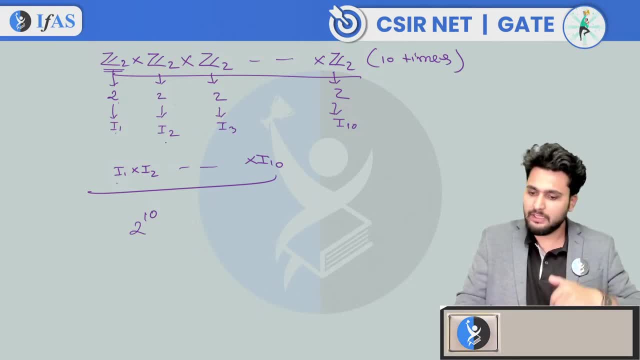 take z2, z2 is an ideal of z2, take z2 instead of i2, take z2 instead of i3, if I take z2 from here, it is an improper ideal. So if we talk about a proper ideal, 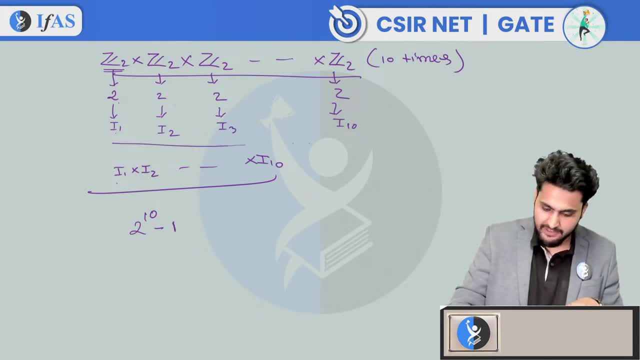 how many choices do we have? 2 to the power, 10 minus one choice. here we have to do less. In this case, all of them are z2, z2, z2.. So how many total choices do we have? 2 to the power, 10 minus 1.. 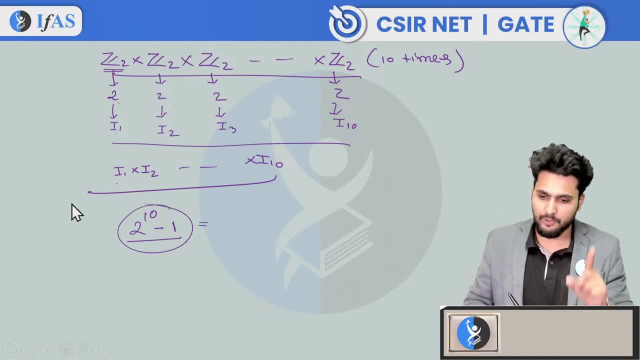 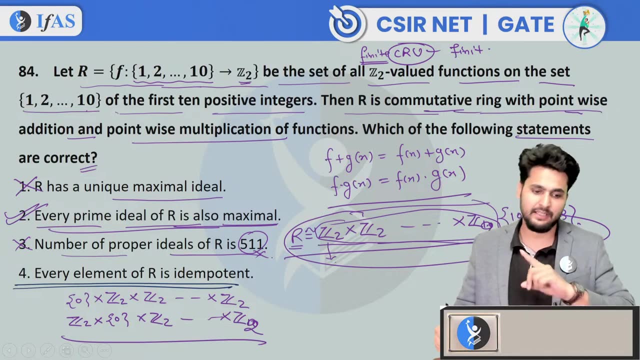 Whatever number comes, that will be the total number of proper ideals of R, Whereas here 5, 1, 1.. 5, 1, 1 will not come for sure. 2 to the power, 10 minus 1.. 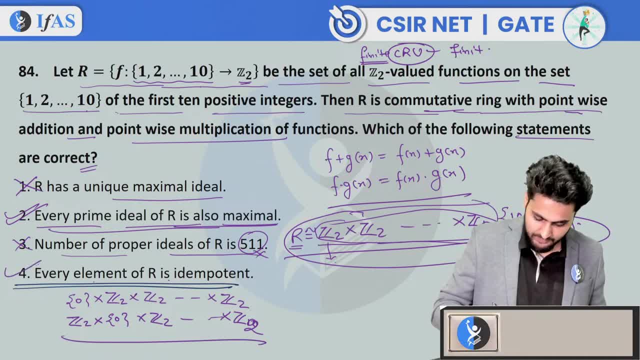 5, 1, 1 will not come. So this is wrong. Every element of R is idempotent. This is also wrong. We know that z2 is idempotent Because z2's every element is idempotent. 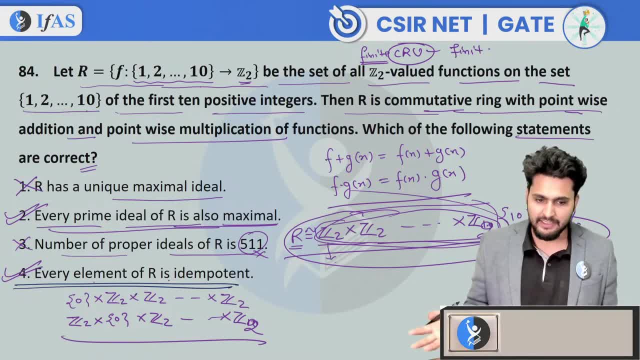 So z2 cross, z2 cross, z2,. no matter how many times you do it, it is always the same. So its every element is idempotent. So 2 and 4 are its correct options, Whereas 1 and 3 are not correct. 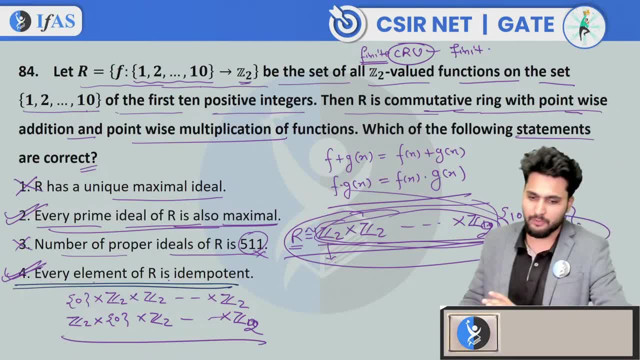 I hope you understood. If anyone has any further problem, then you can ask. I don't remember the year. I think it was asked in 2018.. But it is a very good question. It was asked in 2017.. Let's do the next question. 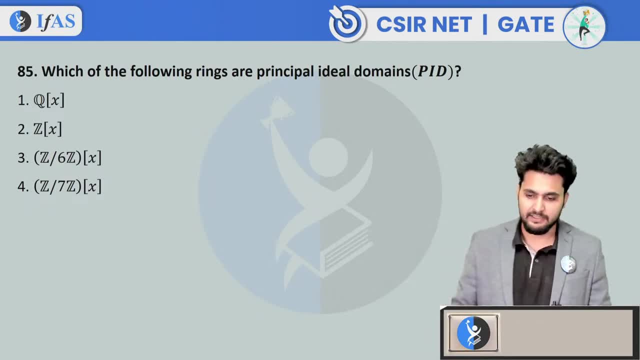 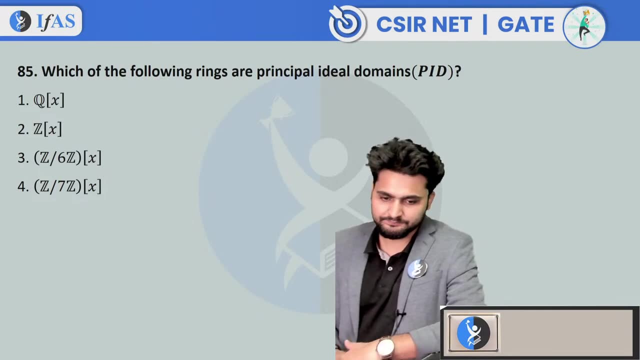 Which of the following rings are principal ideal domain: PIDs. I think you should do this. If you have even thought about it in the last one, then it will be easy for you. If you have even understood the last one, then I think you should do this. 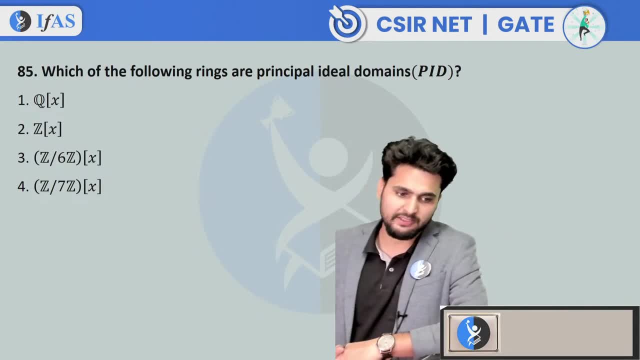 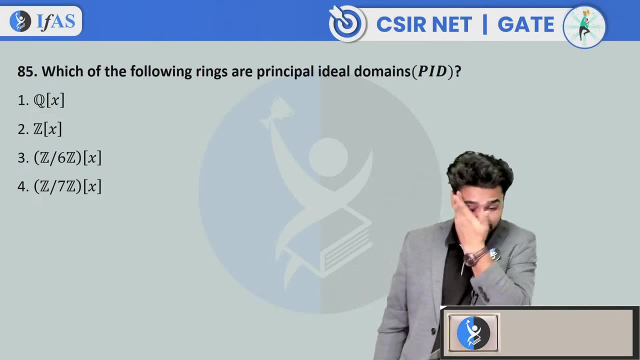 Which of the following rings are principal ideal domain? Which of the following rings are principal ideal domain? Think about it. If you don't know, then don't leave. I told you earlier, If you don't know, then there is something which you have not studied yet. 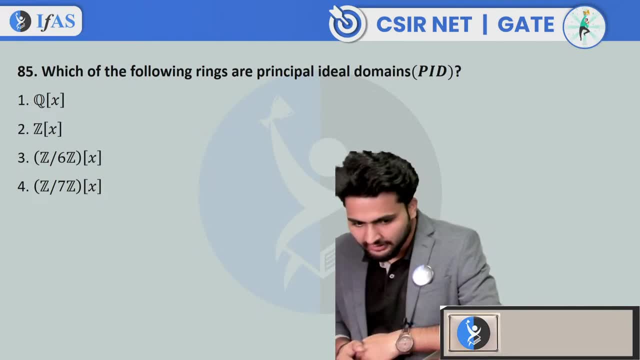 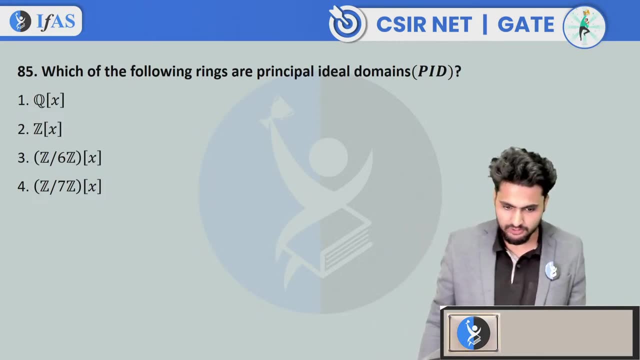 or you are forgetting, It will come to you. You think 1 and 4.. You think A A D, then you think A D. If you think A D, then you should correct D as well. Perfect. 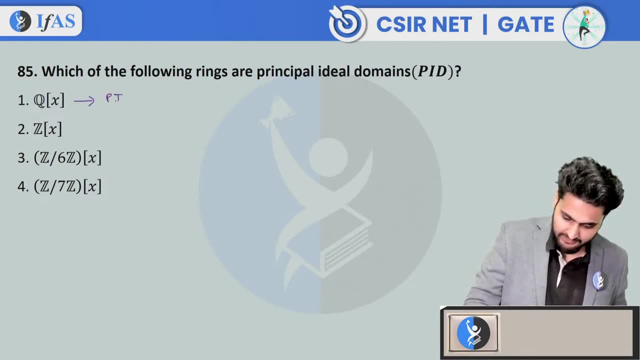 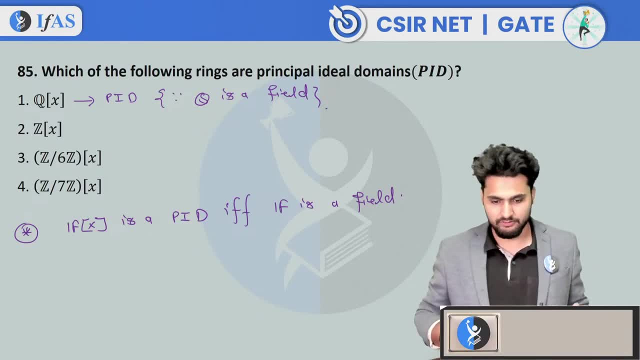 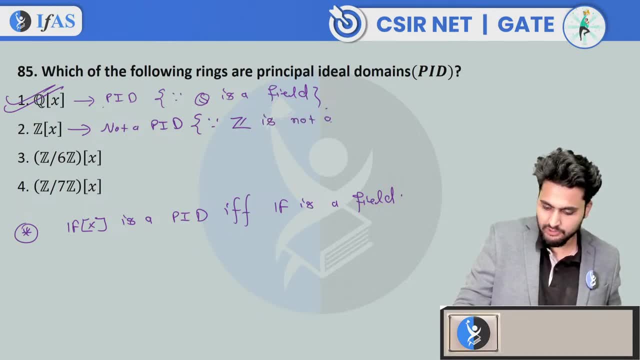 Since z is not a failure, z is not a failure. Am I right or not? So this is not a failure. z is not a failure. zx is not an integral domain. zx is an integral domain. This is a unique factorization domain. 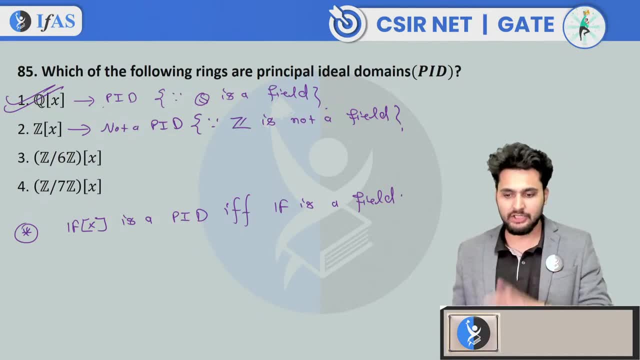 But it is not a principal ideal domain. z still goes up to vmv, Isn't that okay? Z is not your field, So this is not a principal ideal domain. z is not a field. This is z6 x, If I talk about. 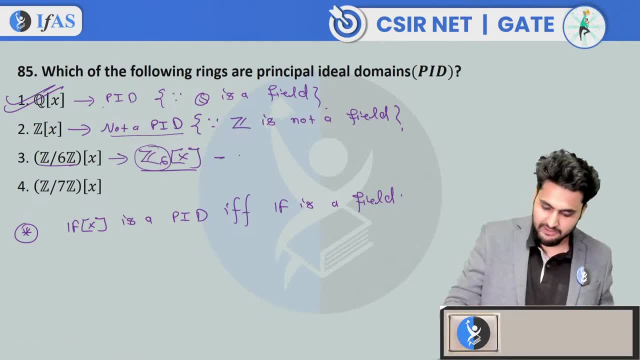 z6x in z6x. So if this is not a field, then we can say it is not a principnl ideal. What does it mean? The reason is that z6 is not a field. Z6 is not your field, Zn is only a field. 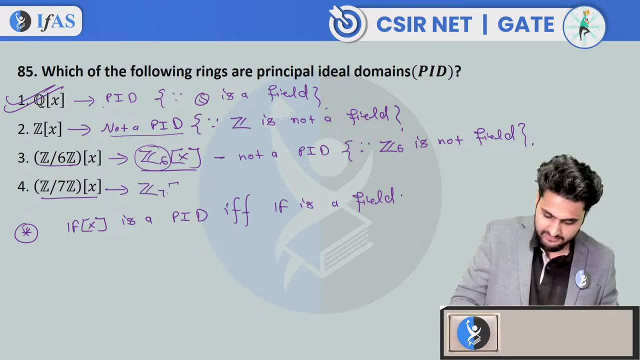 If we talk about this, we will talk about its isomorphism, but this is nothing but our Z7x right. Z by 7 is Z7. Because there is a field next to Z7, so how does it become a principal ideal domain? 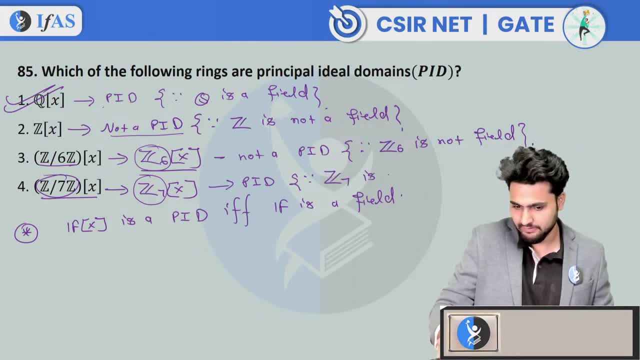 The reason being this: Z7 is a field next to Z7. Is that okay? If someone has some D problem and is not clear in any of the options, then you can answer this question. So which option got corrected? This one and four. they are the principal ideal domains. 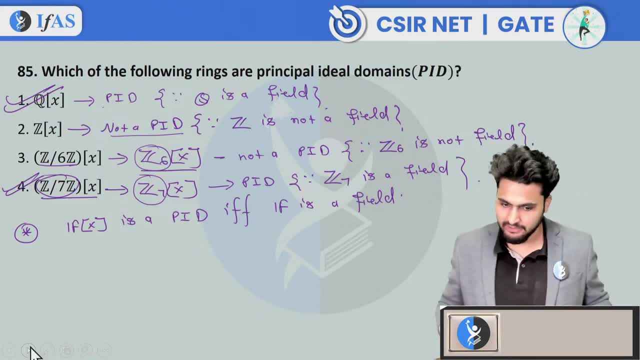 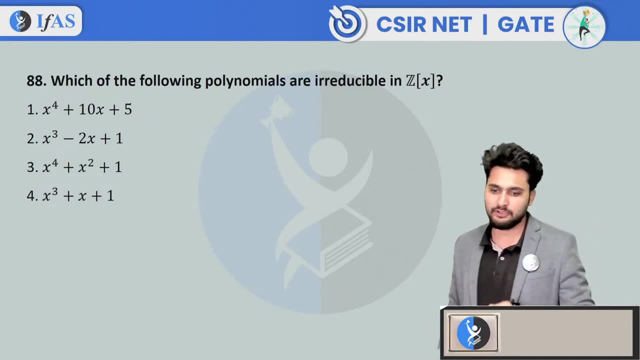 But if someone has some D problem and is not clear in any of the options, then you can answer this question: Which of the following polynomials are irreducible in Zx? Which of these polynomials are irreducible? And I will tell you that I will be uploading a video on irreducibility on this channel today or tomorrow. 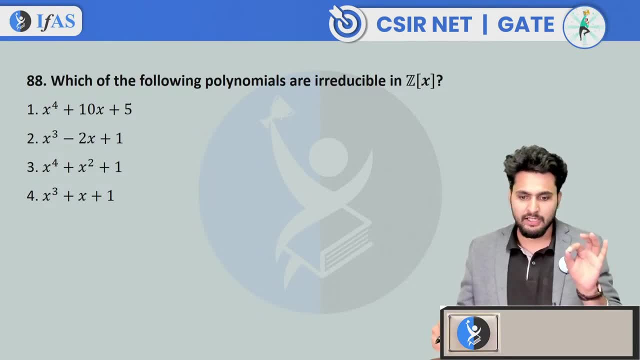 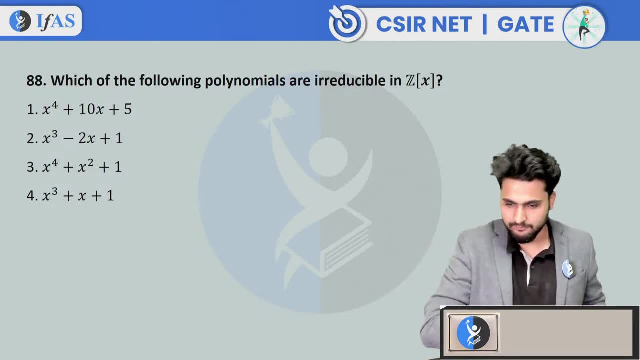 So as soon as it is uploaded, you all have to watch that video. Okay, Okay, that's a very good answer. So now I will tell you the answer of this question. Which of the following polynomials are irreducible in Zx? 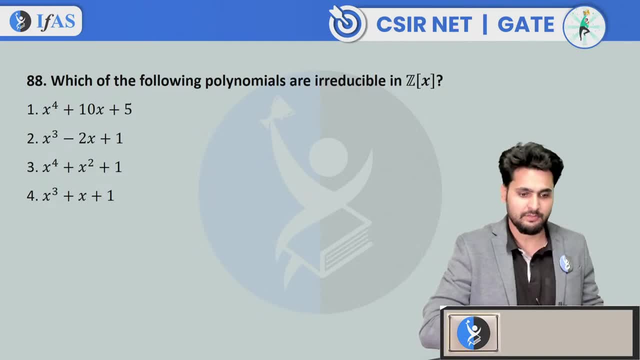 And if you have seen CSI and its previous question papers, you must have understood that there are questions related to irreducibility. Very good questions are asked in irreducibility and quotient ring. Very good questions are asked in irreducibility and quotient ring. 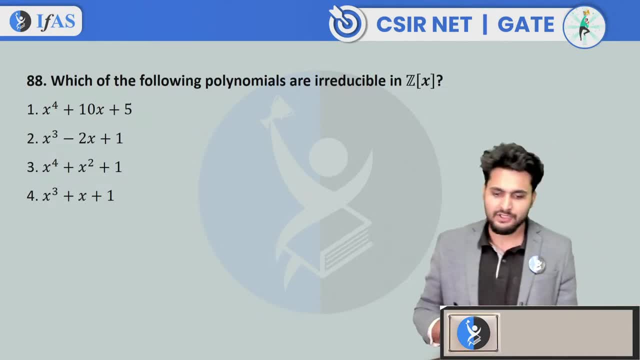 If four questions are asked, if four questions are asked in your exam, if four questions are asked in your exam, then there are three such questions which are usually asked in the quotient ring. Maybe A and B is correct. So, Divyaesh, you think A is correct? 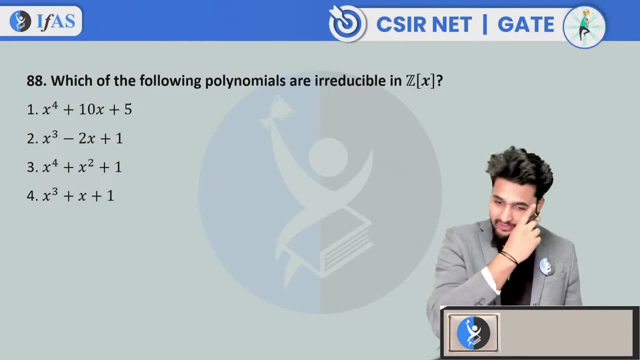 Or you think A & B are correct. So, Chetam, you think A and B are correct. Chetam has her finale, the closing line of A&D. Chetam has her finale, the closing line of A&D. 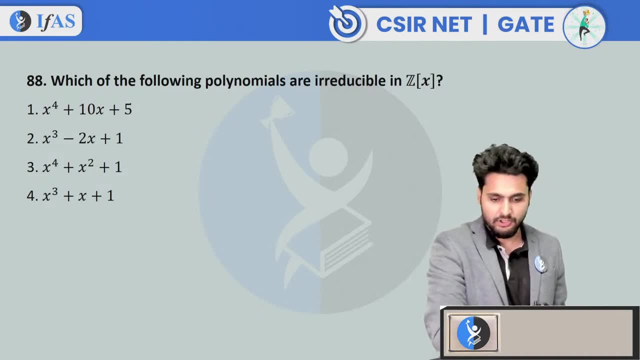 This is correct. A & D are both correct. Divyaesh, I think you did Dchoing, Divyaesh, I think you did Dchoing. And Satna is also correct, And Borissa too, And A&D are the correct options. 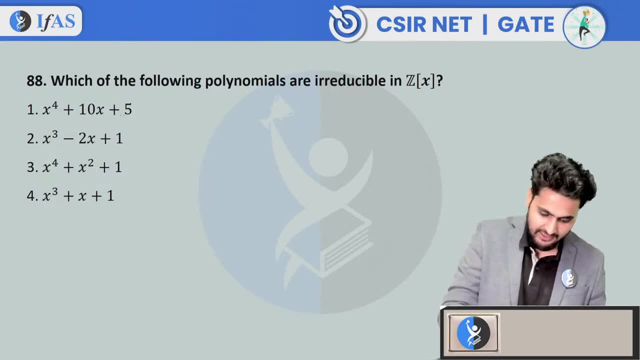 anybody. why do you think first option first is correct? how did you check? what result did you use? tell me anyone wants to know what result did you use that it is reducible in zx. anybody which of the following, which of the following by isis is correct? 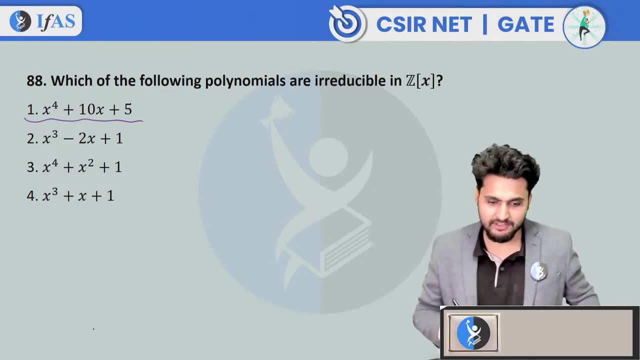 by isis is correct. this is reducible by isis is correct. we can check this. what will we do? in? p equals to: if i take 5, so 5 you divide by this. this is not required. this is not divided. isis takes, isis does not happen. 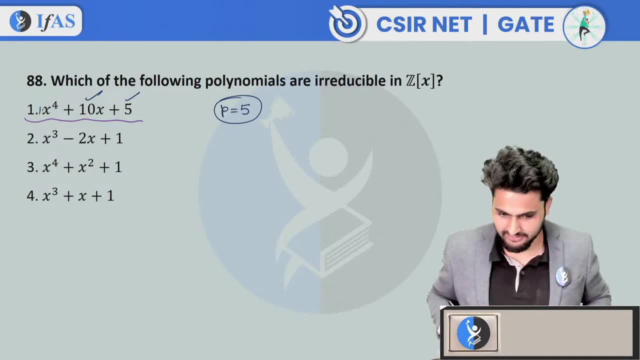 this is e. i says this isis takes for p equal to 5. all the conditions of isis take are satisfied. p squared is 25. that should not be divided. all the conditions of isis take are satisfied. that is why how reducible is is. 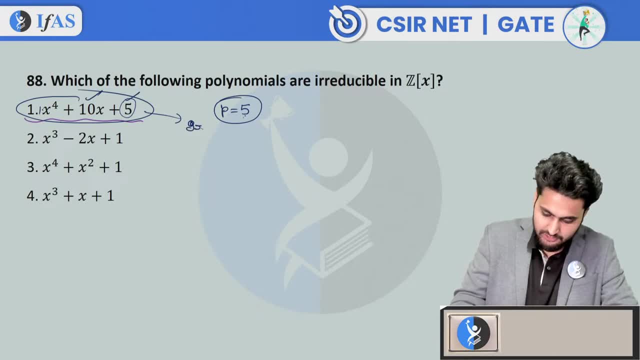 one thing is in q, so this is: is this: Now you will use your common sense a little more, the things you know, you will use it. Now you will understand that, yes, this is irreducible over z. How? Because it is primitive. 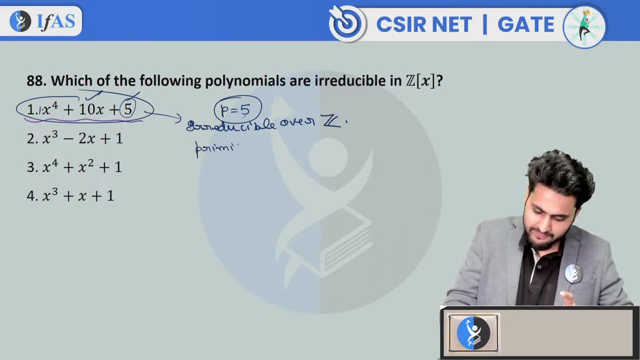 So this is the primitive. You can say primitive or you can also say this: What does primitive mean? What is primitive polynomial? This is the polynomial of zx, whose highest common factor of all coefficients is 1. That is called primitive polynomial. If it is primitive polynomial, then it is irreducible in qx if, and only if, it is irreducible in zx. 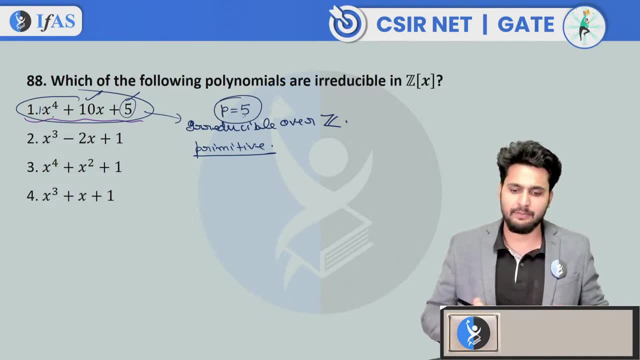 Or you can also say that, apart from 1 and minus 1, if you are not getting any coefficient common in polynomial, then if the polynomial is irreducible in q, then it is irreducible in z as well. So because it is primitive, implies that we will say: this is irreducible over z. 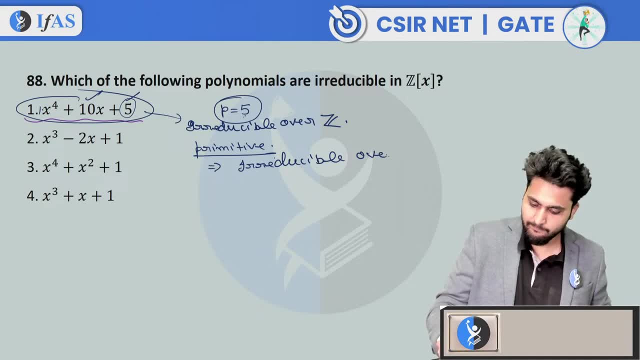 Irreducible over z, So this will also be irreducible over z. so this is correct. If this is correct, then the factor will be easily visible to you. Write x: cube minus x. Write minus x. Write plus 1.. 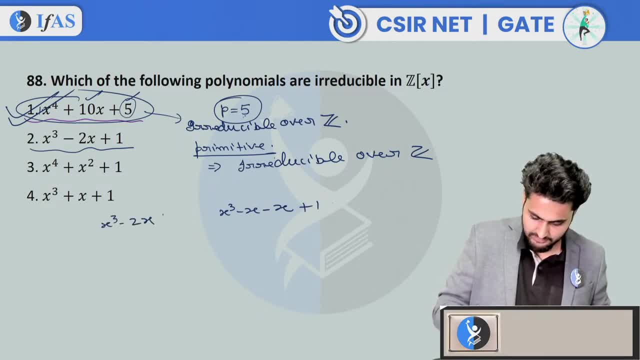 So I have written x cube minus x plus 1.. This is equal to minus x plus 1.. If x is common, then x square minus 1 is left. If minus 1 is common, then x minus 1 is left. 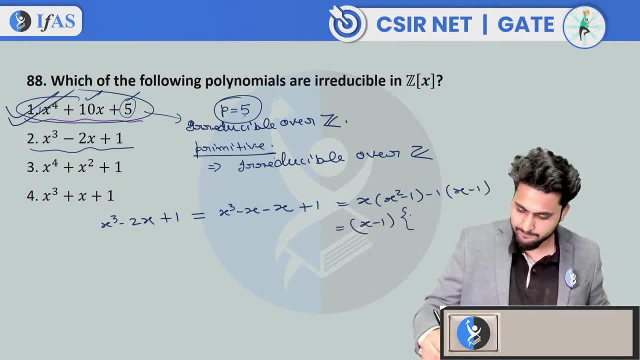 This is equal to x minus 1.. If we do it outside then it will be left x into x plus 1 minus 1.. So it means that it splits into two polynomials of z, Both the polynomials of z. 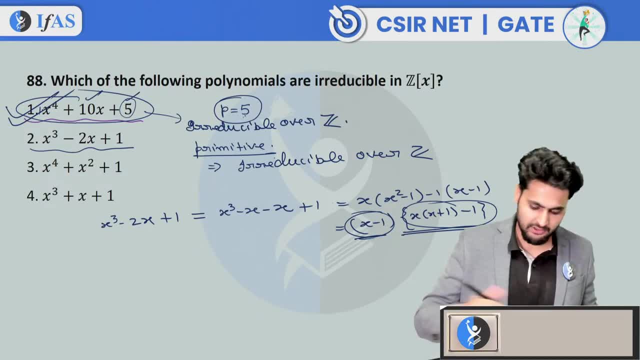 It breaks into two polynomials. It breaks into two polynomials. Both are non-indexed. This also means that there is a reduction. So this is correct: x to the power, 4 plus x, square plus 1.. This is also reduced. 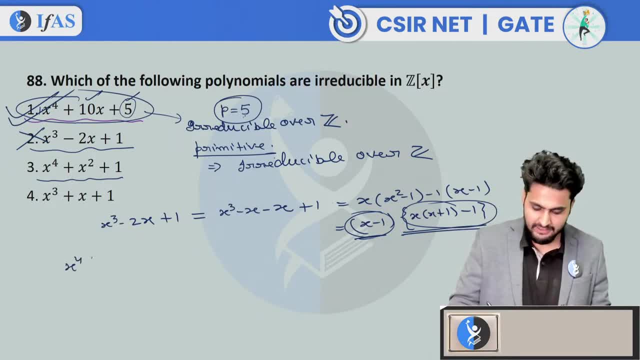 You have to think a little about how it is reduced: x cube plus x square plus 1.. So if you see I write it like this: x to the power, 4 plus x square. I added one, x square, I subtracted one. 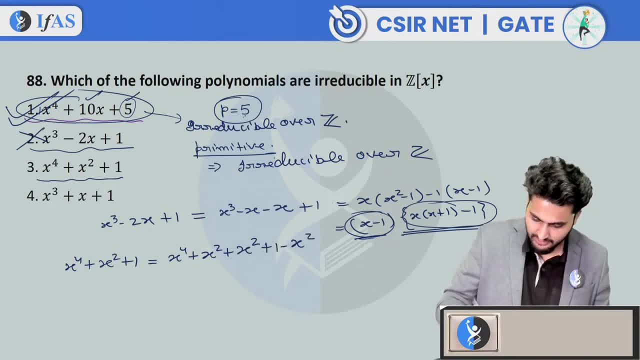 And I will do that later. First I will change it Just 1 minus x square. If you see this, this is nothing but x square plus 1 whole square. Can we say that Minus x square? Now this is equal to x square plus 1 minus x, into x square plus 1 plus x. 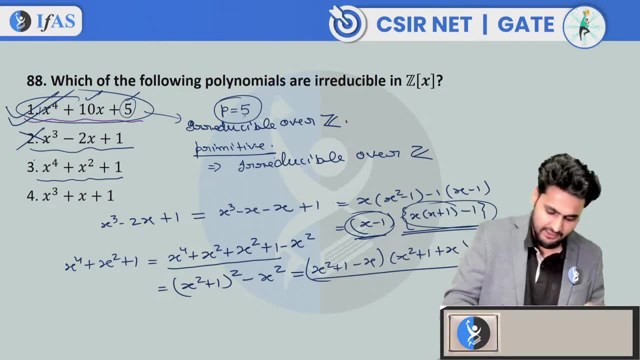 So two polynomials are split. This means that it is reduced, So this is also reducible. What is left? This one? And how will you call this irreducible? Just change it a little bit. What is this? Just change it a little bit. 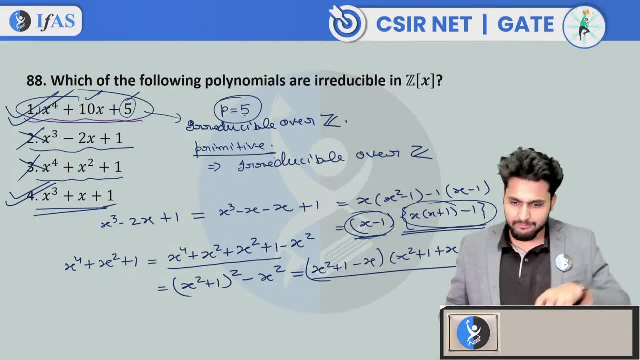 Just change it a little bit. Just change it a little bit First, we will solve it. Anyway, why d4 is the irreducible polynomial. They have answered d, So I will tell you why d. What do you do till then? 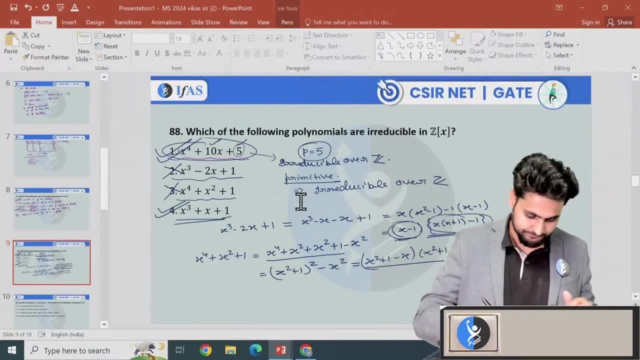 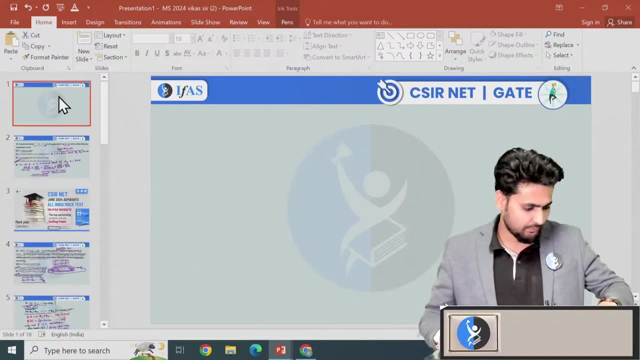 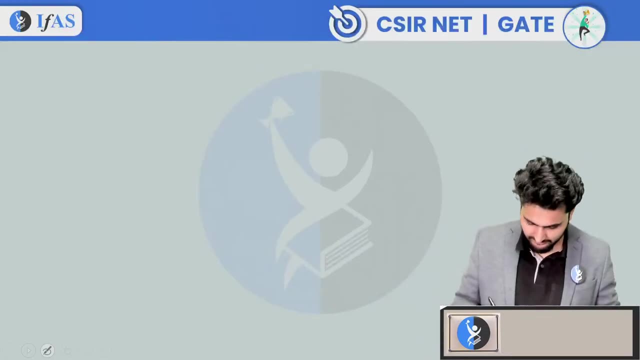 Let's talk a little bit about Einstein's criterion. What is Einstein's criterion? As I told you that I am going to upload a video of 15 minutes, 10-15 minutes on irreducibility. If you see that, all your doubts will be cleared. 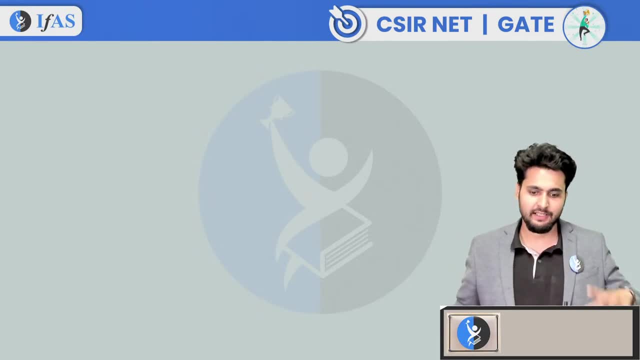 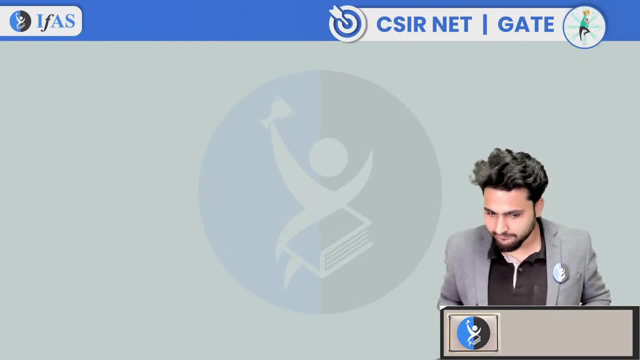 And what did you consider as p, Tell me, For the autopsy? I see a perfect division, which, you are right, Very good. But what do you mean by considering p for the autopsy? Einstein's criterion, Isis criterion, Einstein's criterion? 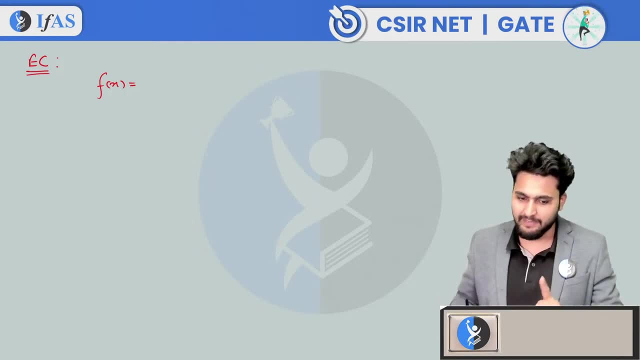 What is it? I have been given a polynomial like this: If only f x is equal to d x. Listen carefully. It is very simple. If you understand it once, that will always come to you. You have been given a question in CSI NET's exam. there are 4 options in it: irreducibility. 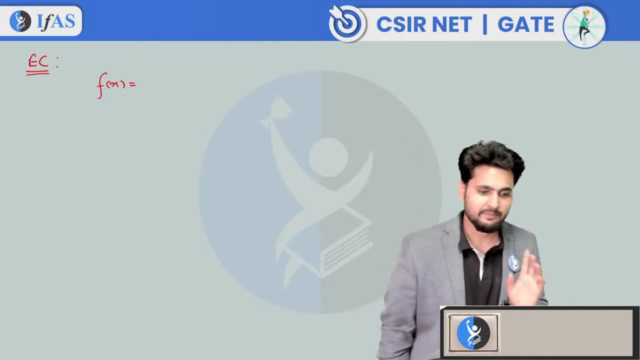 is asked, One option will be guaranteed in which ICS sales criteria will be applied. You can check this in the previous video. P equals to 2. Perfect right. Very good, We will see that right. So f of x equals to- let's assume there is a polynomial given to us, a0 plus a1x, or 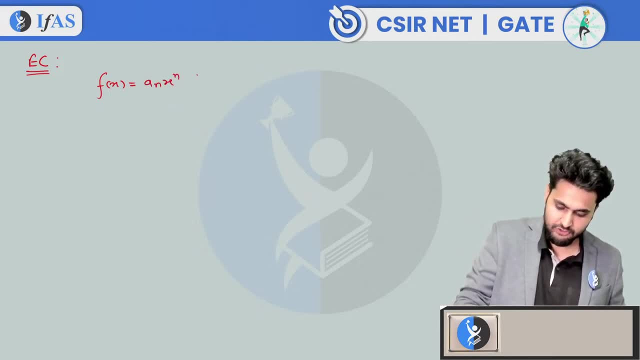 let me write it like this: anx to the power n, a nx to the power n plus an minus 1x to the power n minus 1 plus. let me say a1x plus a0 plus a2x to the power plus a1x plus. 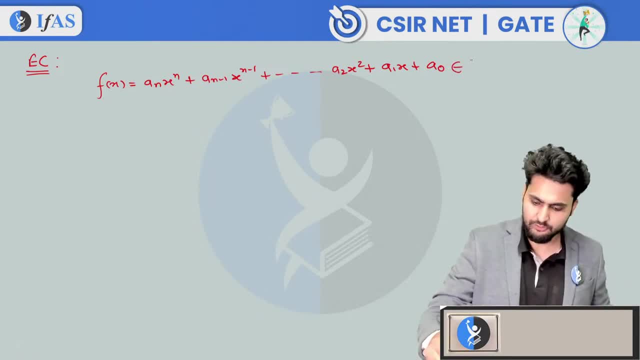 a0. Means you are getting a polynomial of any n degree that belongs to jx. So where will the coefficient go From j? This polynomial f of x is irreducible over q. This is irreducible over q. Irreducible over q. 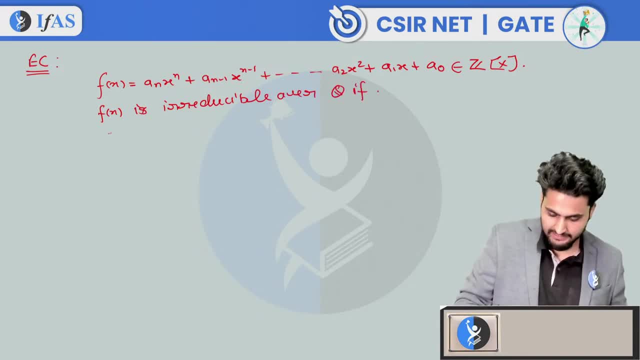 Over q. So when will it happen If? if there exists a prime, there exists prime p, there exists prime p, such that a prime p should exist, so that all these conditions will be satisfied. So the first condition is that p or like this, what condition should be satisfied? 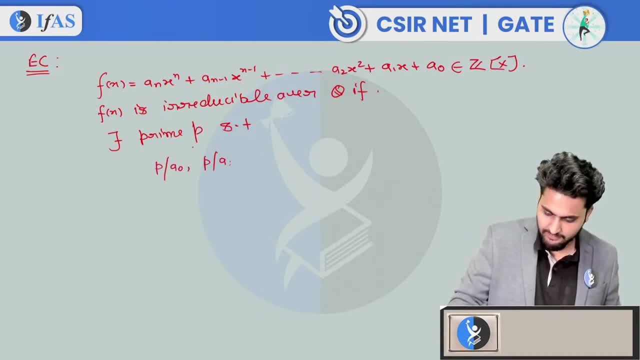 p divides a0 comma. p divides a1 comma. p divides p divides a1 comma. p divides a2 up to p divides a n minus 1.. This is the first condition From this point a0,, a1,, a2, and to this point. 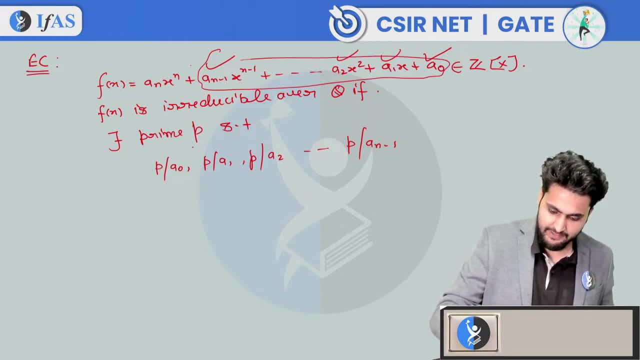 All the coefficients should be divided by p, The first condition. Then what is the condition after that? p should not divide by the highest degree coefficient, p should not be divided by the n. There is another condition. if I do p squared, 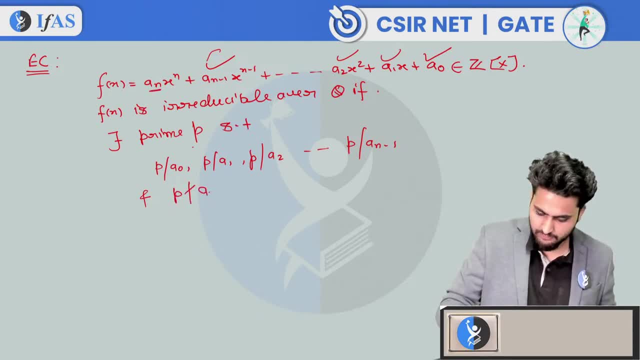 Then what should be done is: the constant term which you have should not be divided by that. p squared should not be divided by a. That's it. If we get any one such prime that will satisfy all these conditions, then our polynomial. 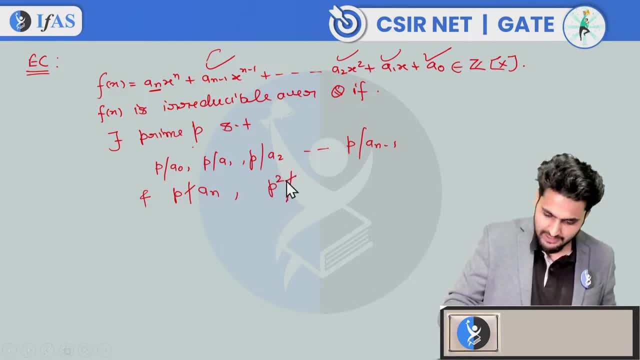 will be irreducible over q, And if you check it here, then you can see that n is irreducible over q. If you check it here, then you can see that n is irreducible over q. That is the condition. Now, what is the condition? 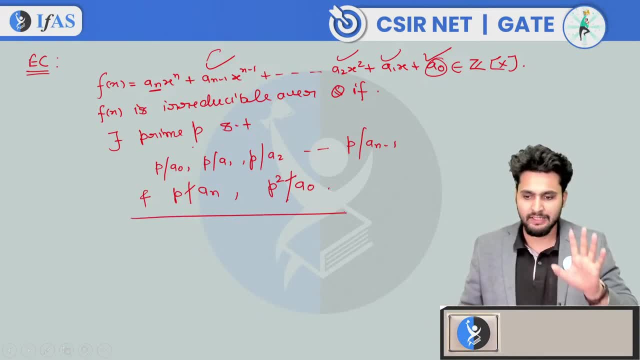 should not be divided. p square should not be divided. that's it. If we get any one prime which satisfies all these conditions, then our polynomial is irreducible over q And if you check here, then we are getting p equals to 5, which satisfies all these conditions. 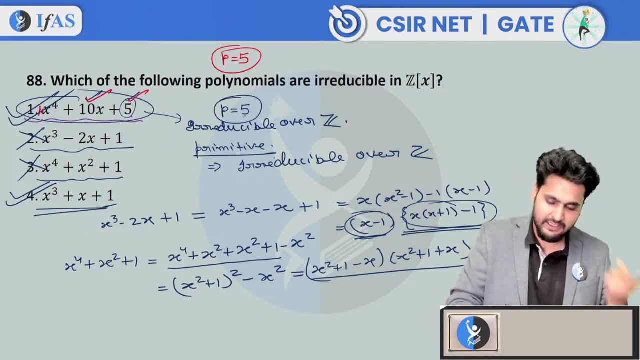 Look, p divides this and this. we should not do the highest degree coefficient, we should not do it. And if I do its square, what will be its 5? 25. So 25 is your high. The constant coefficient should not be divided, we must give it. we have p equals to 5, which satisfies. 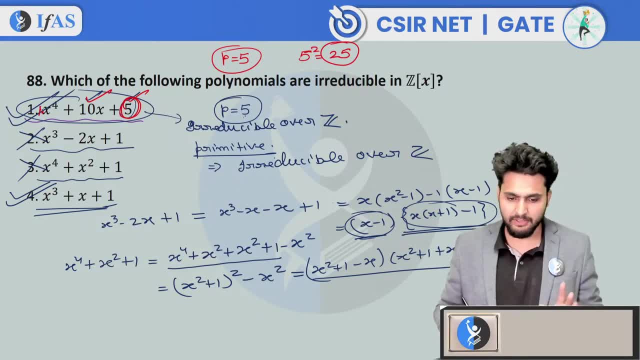 all the conditions. So that's it. So this is Einstein's criteria. Let me tell you. So we were on the fourth option. Why did the fourth option become irreducible By the p test? we can check that, If you see. if you see, how is this polynomial over z2.. This 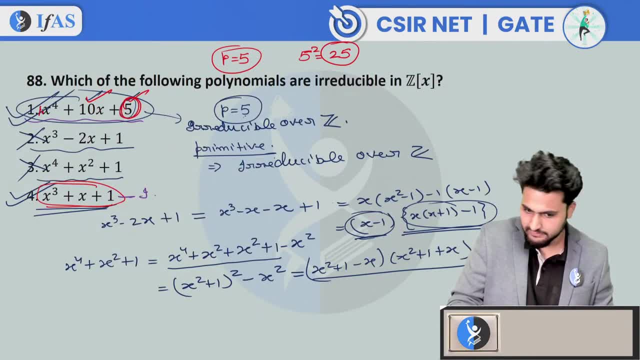 is irreducible over z2.. It says irreducible over z2.. Irreducible over z2.. So the original and what does t test say? t test says that if any polynomial is given to you and you are checking it over q, you don't understand that any prime 3 exists like this. 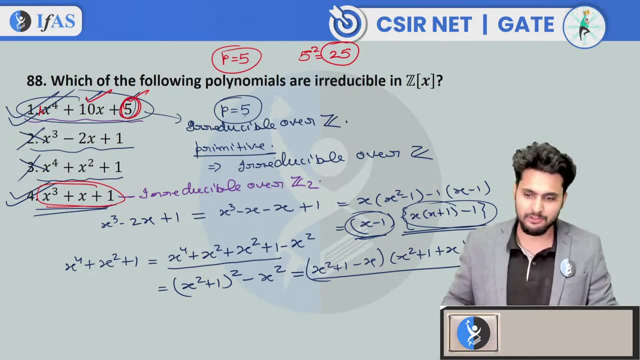 so that that polynomial becomes over zp, it becomes irreducible and the degree of that polynomial, whether you take over zp or over q, should be the same, like if I ask the degree of this polynomial whether I take degree over z2 or over q. it is free and it changes. 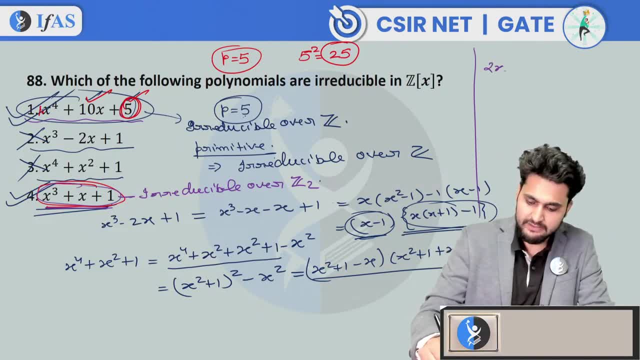 like, if I take a polynomial, let's say 2xq plus x plus 1, if I take this polynomial and ask you what is the degree of this polynomial over q, you answer that it is 3, if I ask you what is the degree of this polynomial over 2?? 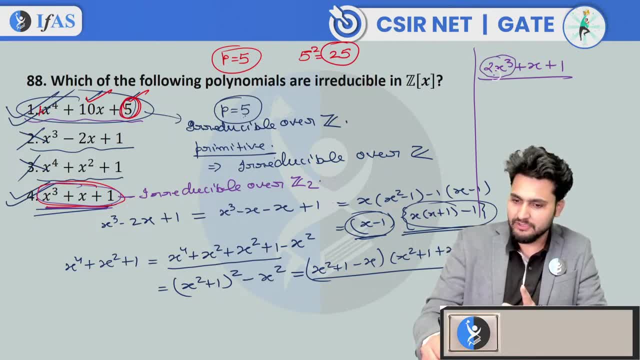 you will see that it is over z2,. so when you will see over z2,, then this coefficient is 0. then what will be the degree of this polynomial? it will be 1, so many times it changes that doesn't happen. 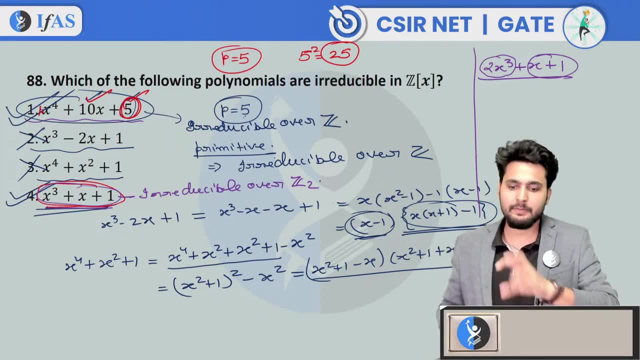 so why do we check? any polynomial is irreducible over q if you see irreducible in any zp. so why is the degree of this polynomial over zp is same, so why will it become irreducible over q? so why will it become irreducible over q? because this is primitive. 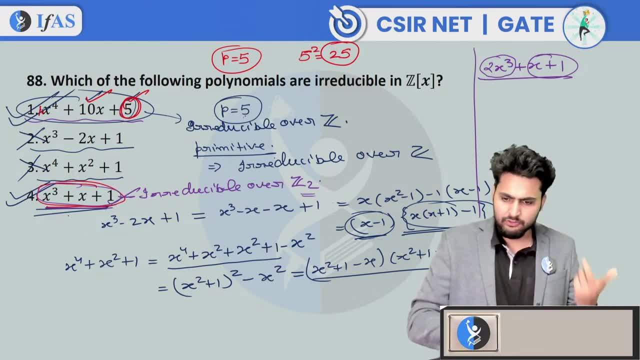 there is no root in this z2,. this polynomial is 3 degrees, so we will do the irreducibility root test. Let's check. there are two elements in z2, 0 and 1. 1 is not the root of this. it is a polynomial of 3 degrees. 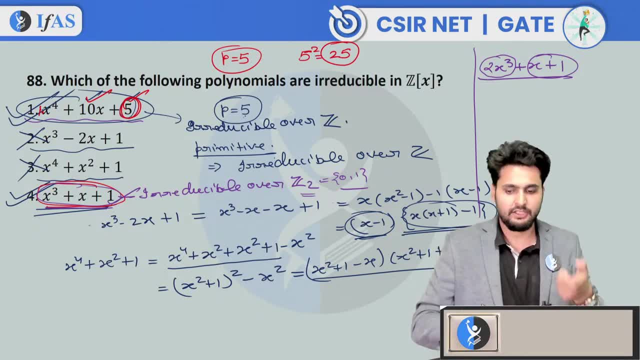 so irreducible over z2 is done. by the way, irreducible over q is done. that means it is the same degree. so why is it irreducible over q? because it is primitive, so irreducible over zp. Thank you so much for watching this video. 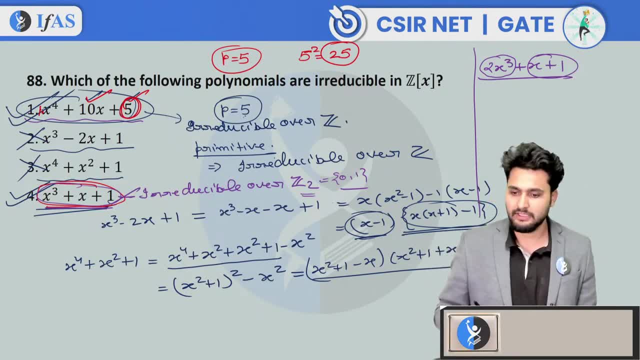 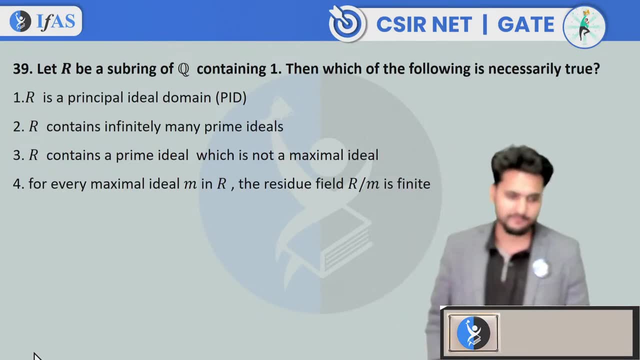 I hope this information will be clear. Let's move on to the next question In the next lecture. tell me what you want to study, Because tomorrow's lecture will not be available. Tell me what you want to study. What do you want to study in tomorrow's lecture? 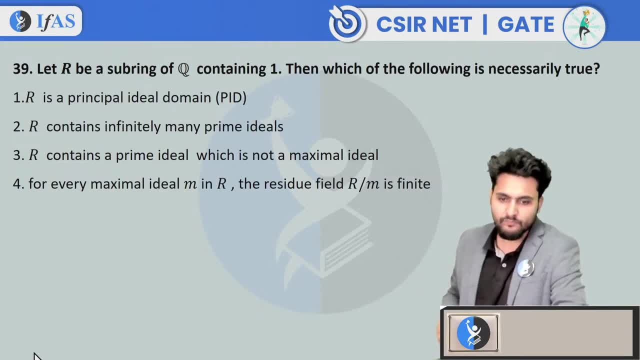 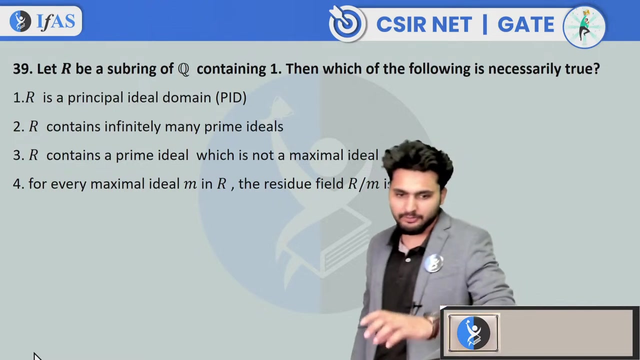 Question number. Let R be a subring of Q, then which of the following is necessarily true? Q R is subring of Q. Q R is subring of Q, which contains 1.. Think about this and let me know. Answer this question. 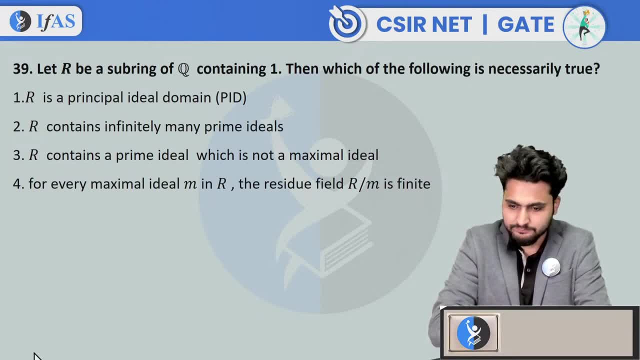 Tell me what you want to study tomorrow. Answer this question. Let R be a subring of Q containing 1,, then which of the following is necessarily true: Q R is subring of Q containing 1,, then which of the following is necessarily true: 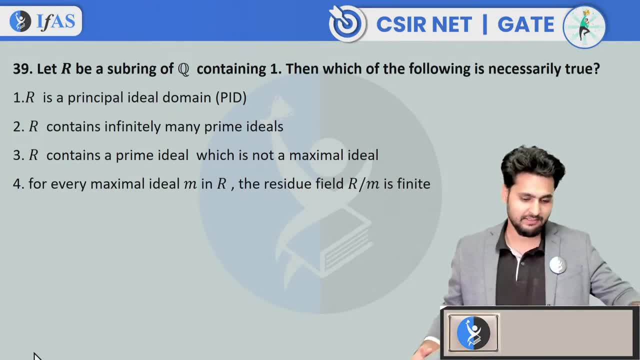 Answer this question. Q R depends on its answer. Answer this question. Q. R is a principally ideal combination. R contains infinitely many prime ideals. contains fingers, Hair, contains cells. correct Versha, A correct and A is correct. I will tell you that it has a very simple counter example. 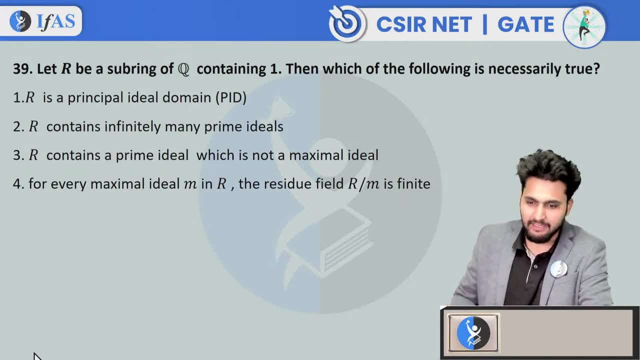 You can discard all options except A. If A is left, then it will be correct. For which example You can consider a trivial subject, Trivial subject or correct. I think trivial is the way to discard your subject. R contains infinitely many pri. 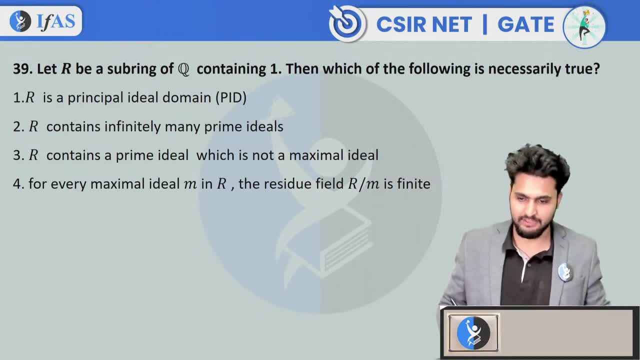 Or I think Q can be considered Not trivial, you can say improper. I have been told that R is a subring of Q containing 1.. I can take Q as well. This is a subring of Q Which also contains 1.. 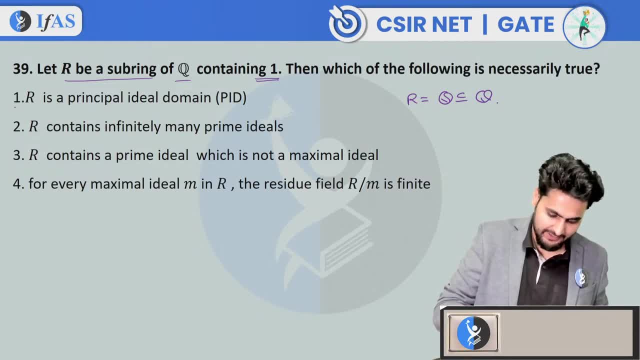 This is also a subring. Q is a subring of Q. Let's do it one by one First. let's do it on this side. Let's start with 2.. R contains infinitely many prime ideals. It is wrong. 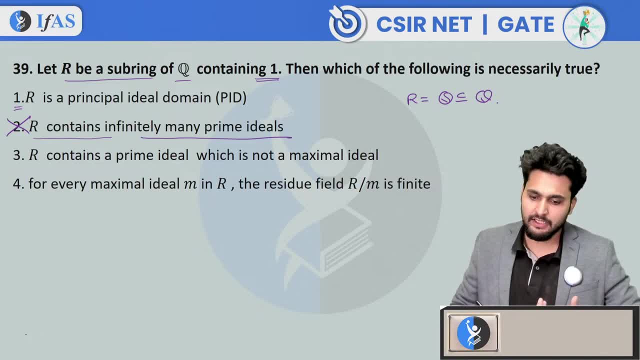 Q has infinitely many prime ideals. It has only two ideals. One of them will be prime. It is wrong. Next, R contains a prime ideal which is not a maximum. This is also wrong In a principal ideal domain. every non-zero prime ideal is a maximum. 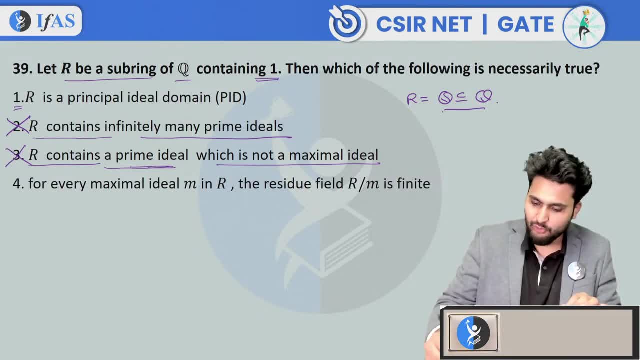 This happens Here. prime is mentioned. If you look at Q, here it has only two ideals. One is zero. This is Q. This is your guess. This is a prime and a maximum. also, This is neither your prime nor a maximum. 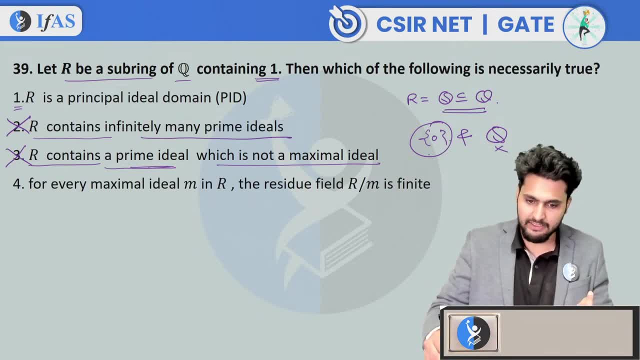 If any Q has a prime ideal, then it is not a maximum. This is wrong. This is also wrong. Next, For every maximal ideal M in R, the ratio R by M is finite. This is wrong. This is a non-zero prime ideal. 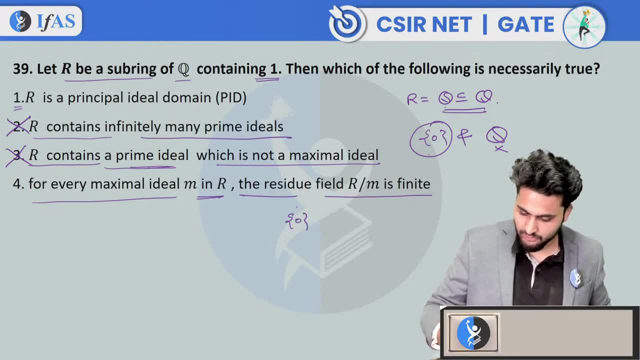 If I take a zero ideal and I say that R contains zero, then Q. If I make Q by zero, then whose isomorphic is this? What is its isomorphic? This is R prime. This is R prime. All these can be your discards. 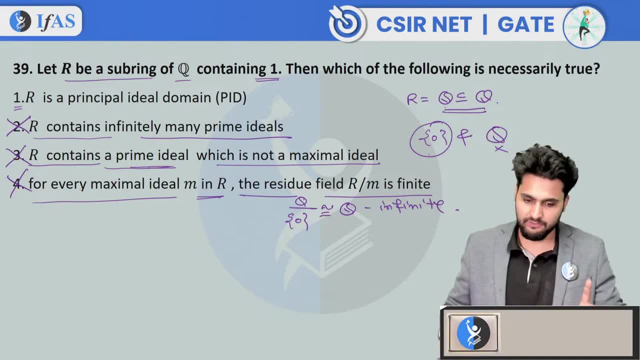 If I take R as Q, Q is a subling of Q which contains two R. All these can be discarded. All this is wrong, So one is correct. I will not prove this. If you are interested, you can do it. 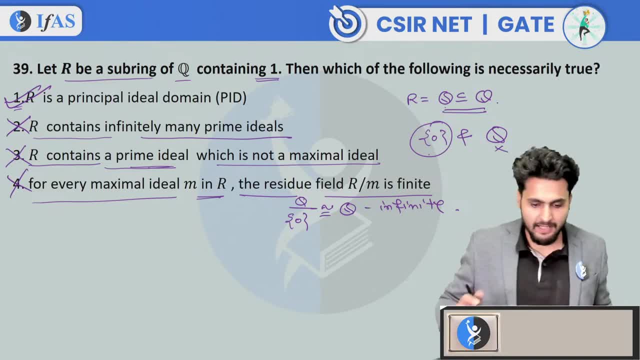 If you want, you can ask me- And you can try it yourself- What to prove. What do you want to prove? If I take a subling of Q which contains one, then it is not a principal ideal. It will be interesting for you to verify. 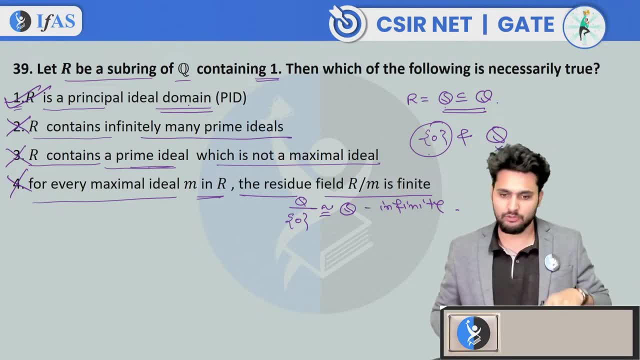 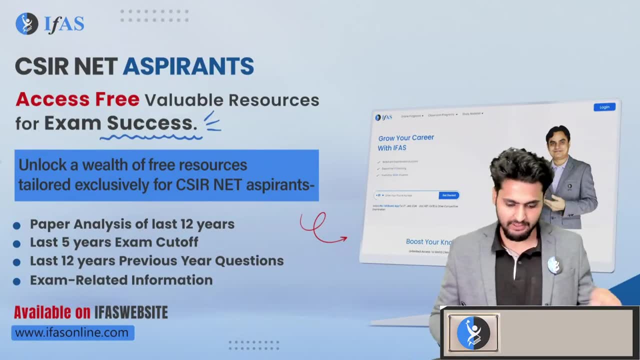 If I take a subling of Q which contains one, then you will have to try it. It is not a principal ideal. You can try it And if you are interested you can tell me. We are friends If you are preparing for NIT. 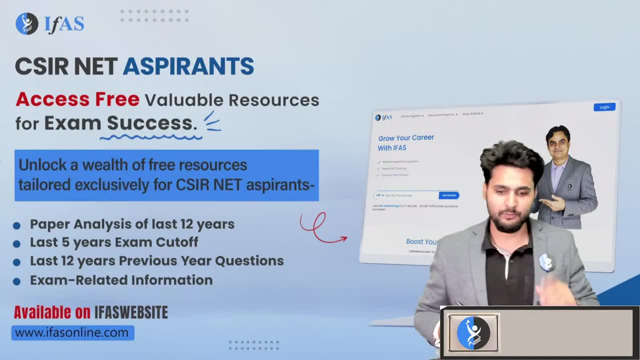 and you have not yet visited all the online websites, then you should use it. There are many such things available. From the point of view of the exam, it is very helpful for you. For example, paper analysis for the last 12 years. 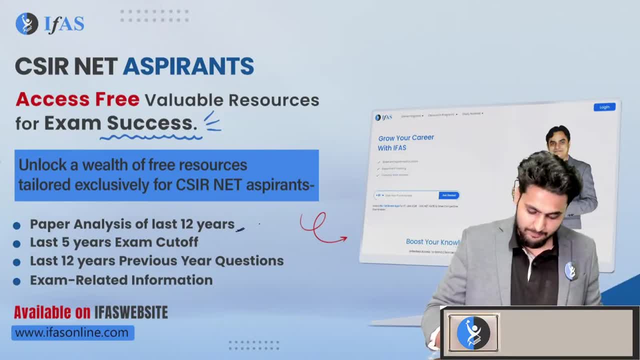 We are still in the 12th year. Paper analysis is available for all of them. How much was asked? from which topic? The cut-off of the last 5 years is available. You can see the cut-off, which will help you. 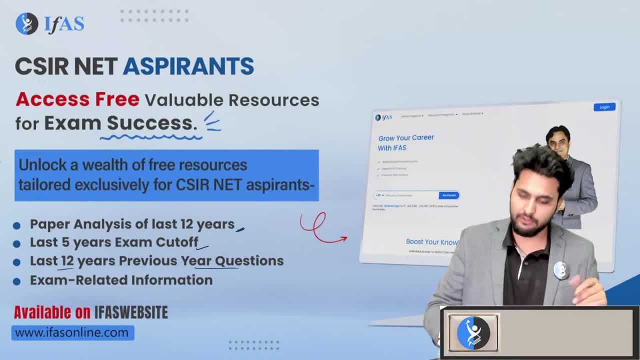 Last 12 years previous question paper. you will get it at one place. You can download it. All exam related information is available. You can visit the IFS online doctor's website. You can visit it. You should make sure that you have this permission. 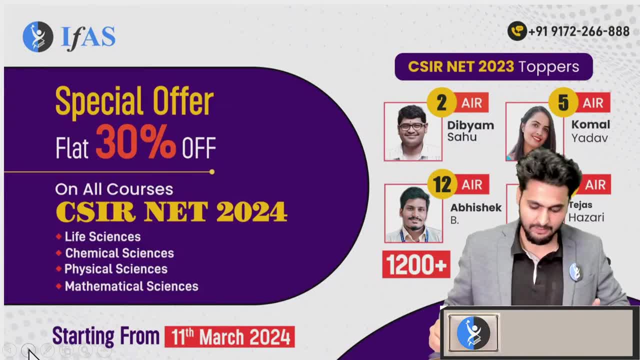 Along with that, CSI NIT 2020,, whether it is June or December, if you are preparing for it, then from 11th March your new batch has started. If you are interested in preparing for it, then you can enroll with 30% off. 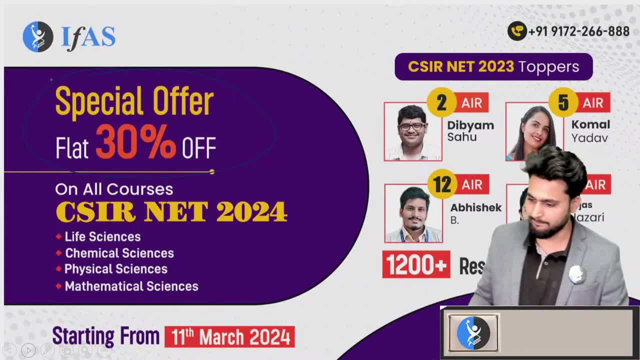 IFS 30,. you have to use the promo code as soon as you enroll. Okay, The site is written here. The site is showing you IFS 30.. Okay, Let's do the next question, And the answer to this is: 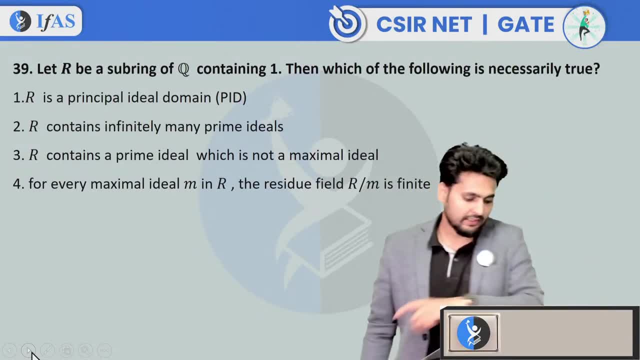 what is it? Look and understand. What is the question. Like the RBA subring, I think we have done this. We have done this. This is not the question. This is also a very good question And this is very simple. 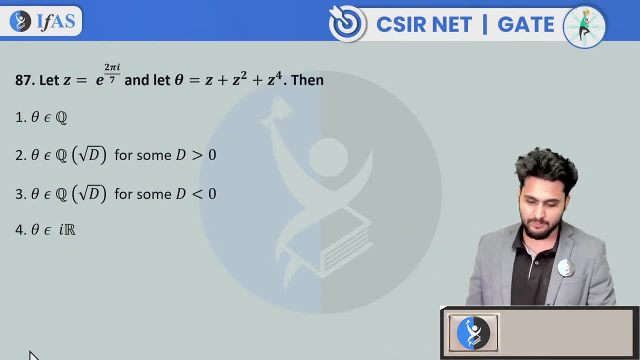 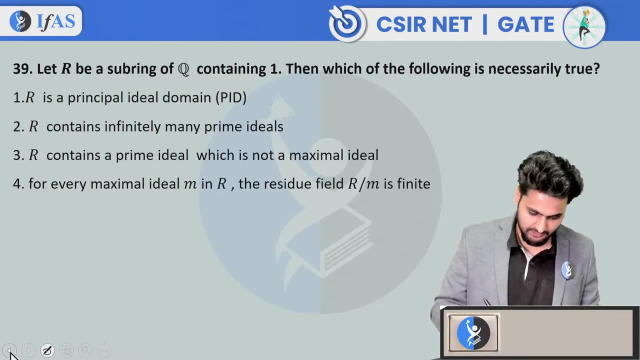 If you have seen it for the first time, then you must have skipped it. Look The last option. repeat this. Okay, The last option. What was the last option? The last option was this: For every maximal idea M of R. 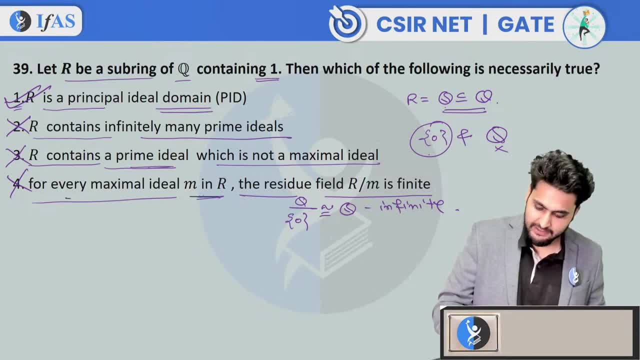 the ratio R by M is 5.. What did you consider R? You have taken Q only. What is R? It is the subring of Q, which contains one. So I have written Q only. What is R? Q? 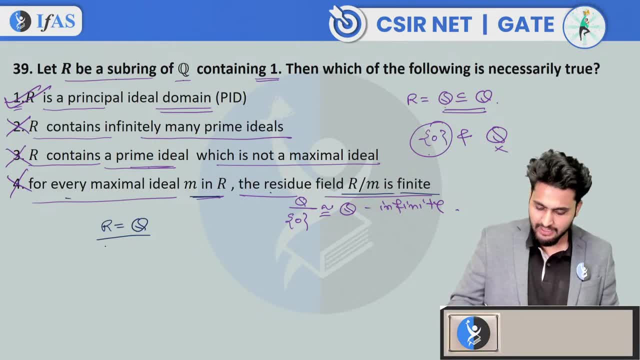 What is R Q? What is R Q? Zero is the maximal ideal of Q. Zero is the maximal ideal. We all know this right. It is the zero is the maximal ideal of Q. Why is it a maximal ideal? 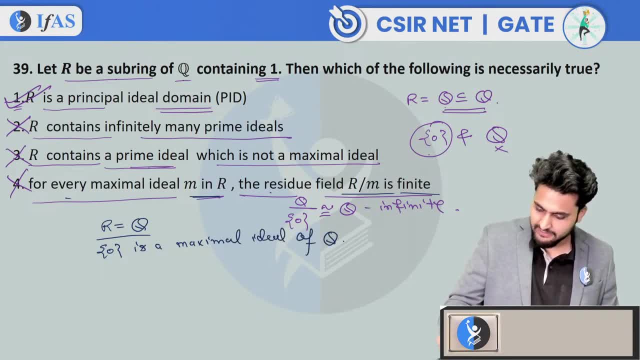 Because there is no other ideal which contains it and that is why it is maximal. So if I make a question string from this: Q, Y, 0.. So it is saying that the ratio R by M is will be finite. 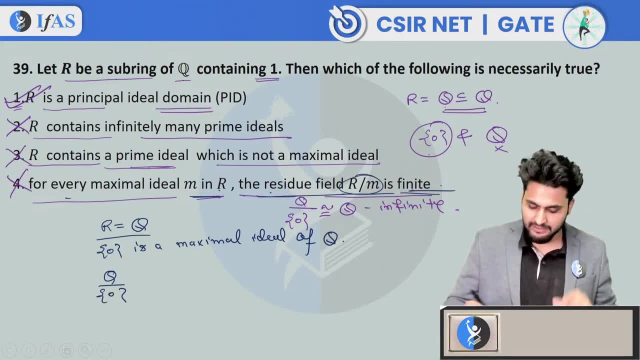 So it is finite. Q Y 0.. This is infinite. This is QK. It is an isomorph, This is an isomorph Q. Correct What is F? It is infinite. So Decidual field or quotient field, which is infinite. if it is not infinite, then this is your discount. 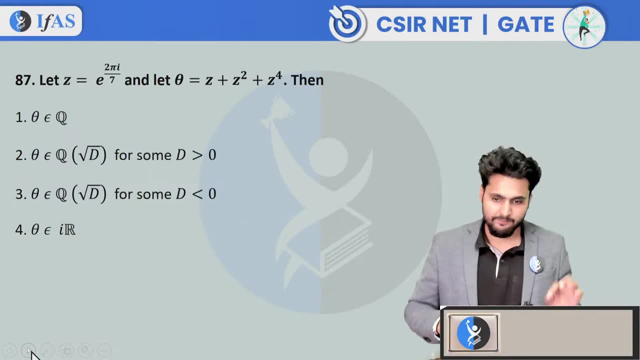 Now tell me the answer to this. This is a very good question. If you have not done it, then don't leave. If you are having difficulty, then also don't leave. We will discuss. When we discuss then also, What is your set e to the power 2 pi i by 7.. What does it mean? 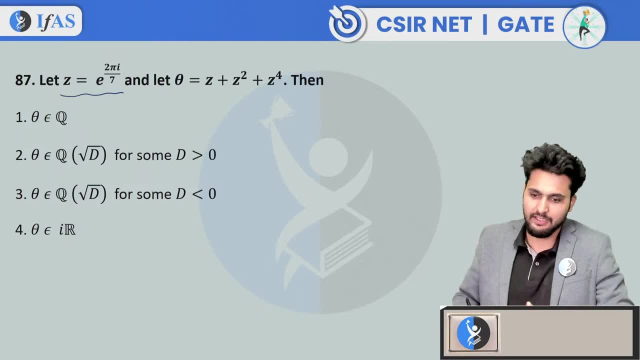 7th root of unity. This is primitive 7th root. Why is it primitive 7th? Because before 7, this power will not give you 1. It is generated. here All the roots of 7th root of unity can be generated. 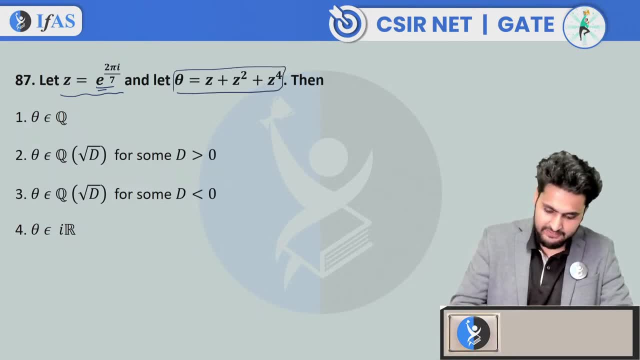 Theta is defined in this way: z plus z, square plus z to the power 4.. Then you have to tell where is the theta member. Is it of Q, Or is Q square root D for some D greater than 0? Or theta belongs to Q square root D for some D less than 0?? 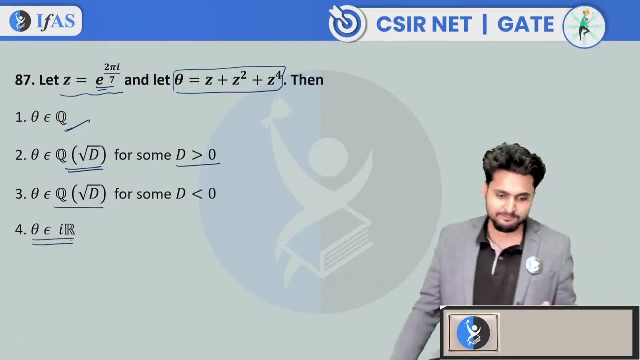 Or theta belongs to IR, Versha and Kalish. do you think B is correct? Tell me more. It is simple, It is a very simple question And this kind of calculation has to be done, Nothing else. Let's see. 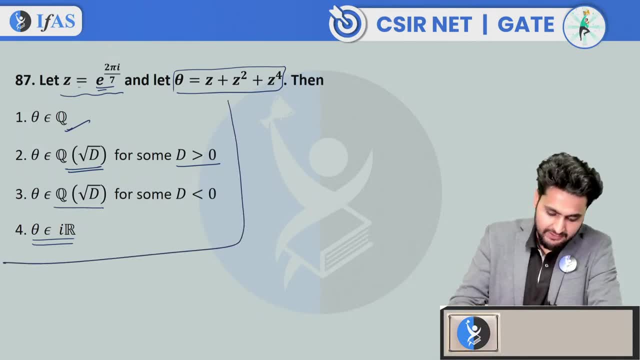 If someone knows, then at least he will understand What is given about z. z is 7th root of unity. Is it primitive 7th root of unity? Shatyam, you think 2 is correct. We will see that 2 is correct or not. 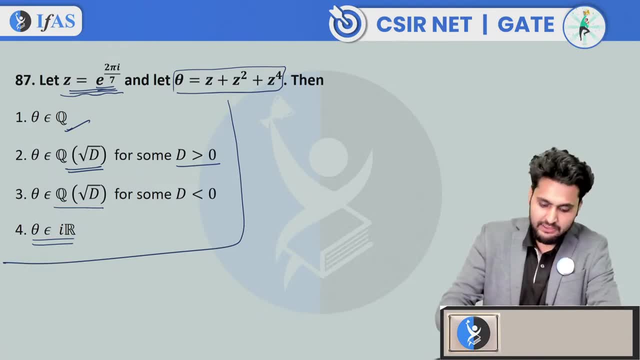 Let's see. So what is given to us is that theta is primitive. Sorry, what is our z? Primitive, 7th root of unity? If there is any nth root of unity, omega, then what condition does it satisfy? Omega to the power? n equals to 1.. 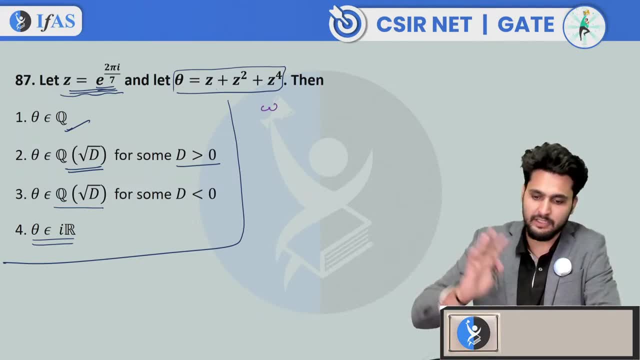 And 1 plus omega plus omega square up to omega to the power n minus 1 equals to 0.. Can we say that? So z will satisfy two conditions. One is z to the power 7 equals to 1.. And z to the power 7 equals to 1 plus z to the power 3 plus z to the power 4 plus z to the power 5.. 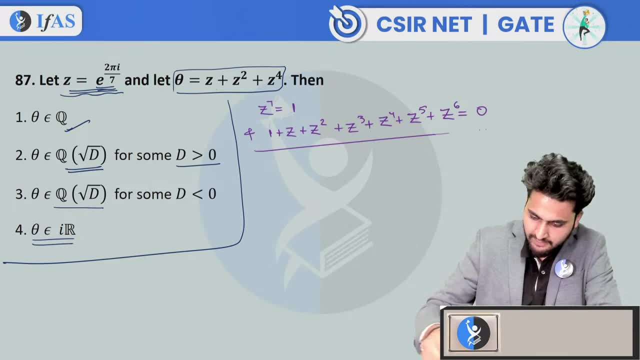 And z to the power 7 equals to 1, plus z to the power 6 equals to 0.. Can we agree with me? Are these two conditions satisfied? Yes, because there is 7th root of unity And z is a primitive 7th root of unity. 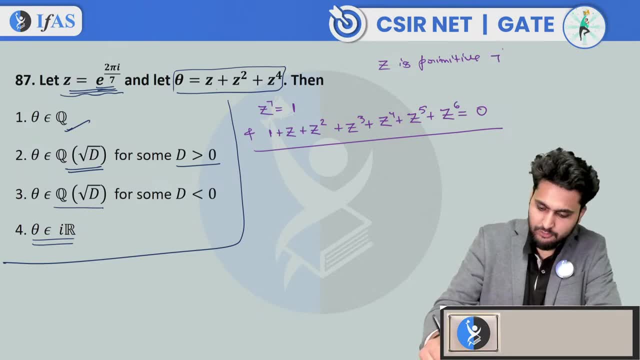 7th root of unity. Is that okay? So this condition will satisfy you. This is a very good thing. Now, what do we do about theta? We spare on both sides. theta is square. and what will happen to it? z plus z- square. plus z to the power, 4 is square. 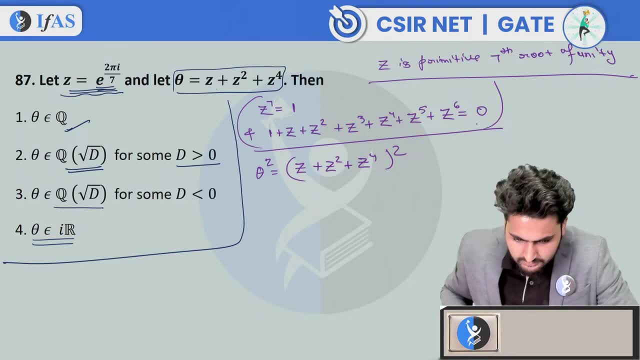 Now we will use it on both sides. What will happen to all the mixtures? So what will happen to theta z square plus z to the power 4 plus z to the power 8 plus 2z, cube plus 2z to the power 6 plus 2z to the power 5.. 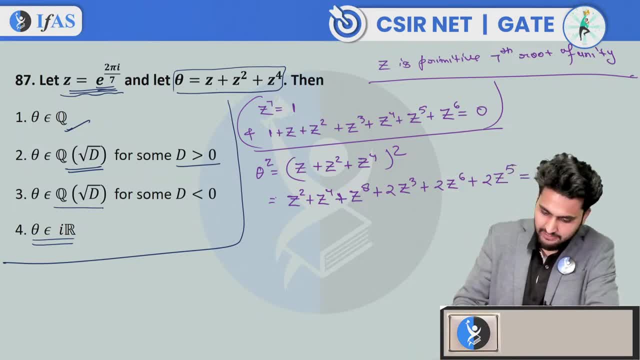 And this is equal to 0.. What is given here? Sorry, this is theta square. theta square is equal to z, So theta square is equal to. What do we do? theta square is equal to. Let's do a little manipulation. 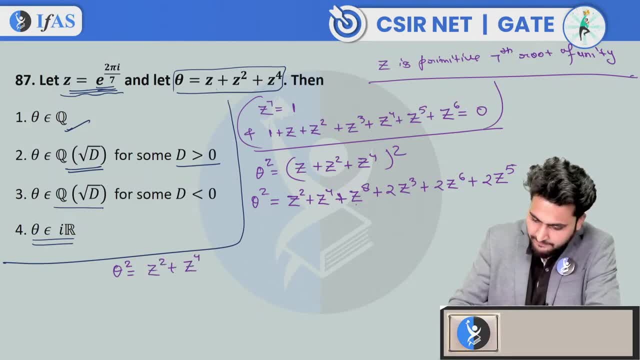 z square plus z to the power 4.. Let's keep it like this. What do I call z to the power 8?? Because z to the power 7 is 1.. So I call it z. What to do? Please tell me how to do it. 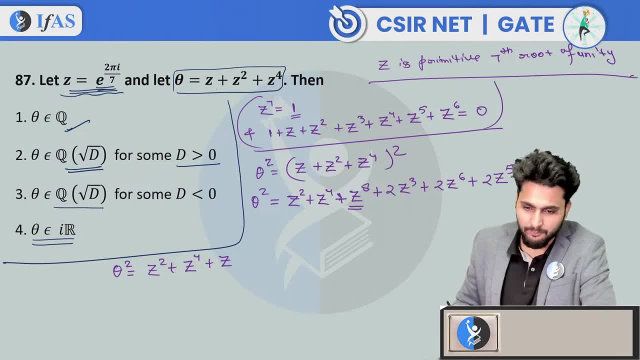 What is happening to all the mixtures? All the things are being studied, All the topics are being studied. It is getting mixed up. Let's do it like this: Give some time to one topic first, Practice the question. One topic. well, 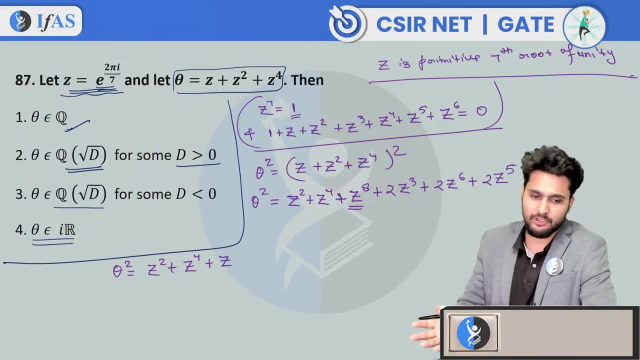 What to do. Do it well. At least one topic will be good, Then you will die in the other. Work hard on one topic first, Then the other will come. There is no time now. You have to do everything after the exam. 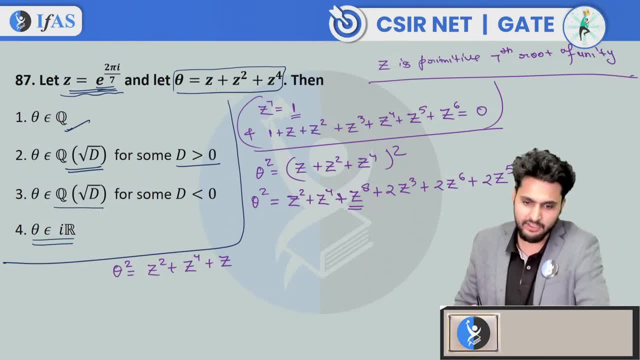 So why do you have to mix it up? It is happening because you are doing it. Okay, Got plus z. Now what to do after that? Take out all of them one by one. If you take out two, then take out one by one. 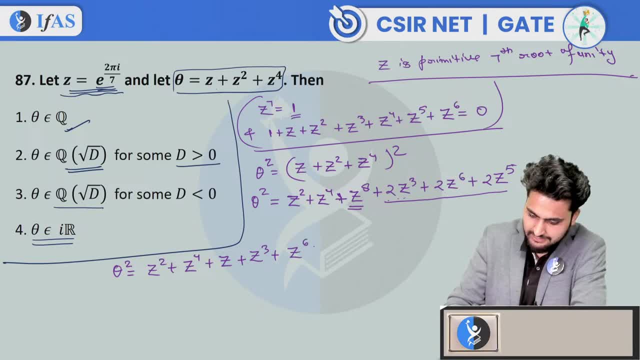 I took out z cube one by one. One we took out z 6.. We took out z5 one by one And I got one by one One. add also One by one. I added One subtracted And the rest which is left. 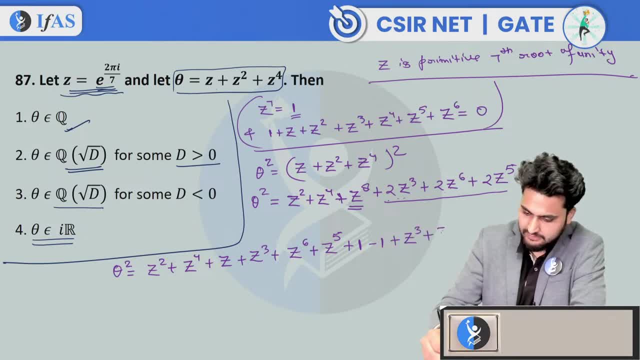 I wrote them down: Z cube And plus to the power 6 and plus to the power 5.. Someone have any doubt? So look this next One: plus z, plus z square, plus z cube, Plus to the power 4, plus to the power 5.. 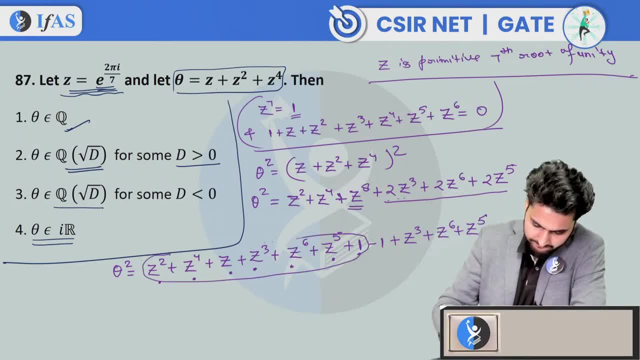 plus z to the power, 5 plus z to the power 6.. I will write this as 0.. So theta square equals to zq plus z to the power 6, z to the power 5 plus z to the power 6.. 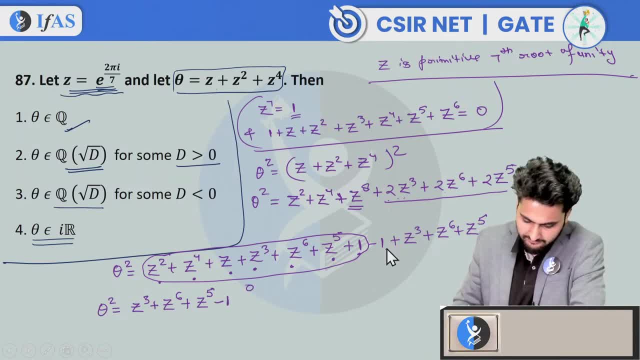 5 is left and minus 1 is left. Now, if I take out the value of these 3 from this equation, then theta square equals to z to the power, 5 plus z to the power, 6 plus z to the power 4.. 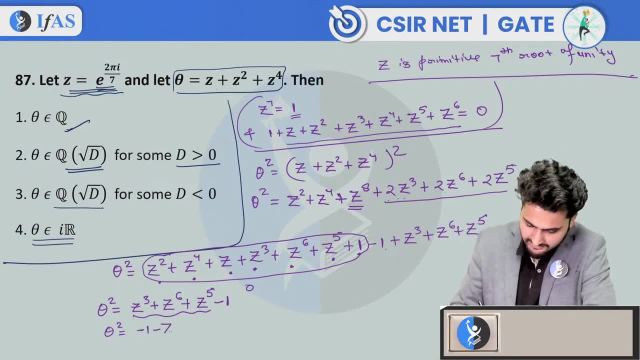 So minus 1 is left and minus 1 is left. minus z to the power, 5 plus z to the power, 6.. minus z to the power, 4 minus 1.. If I take out the value of these 3 from this equation, 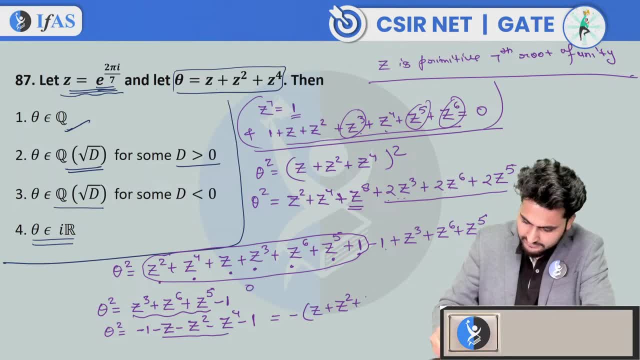 then z to the power 4 plus z to the power 5 plus z to the power 6.. And what else is left? Minus 2 is left. If you don't know anything about this, then you can ask me: What is this? This is nothing but theta. 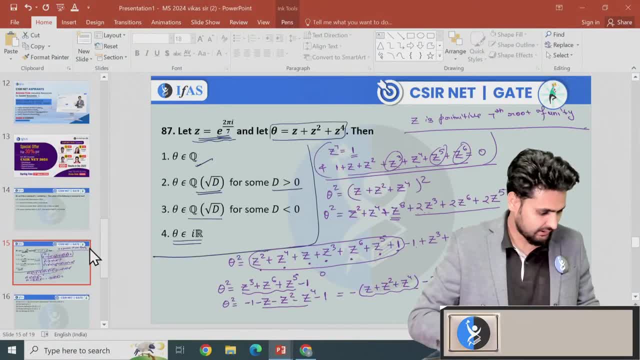 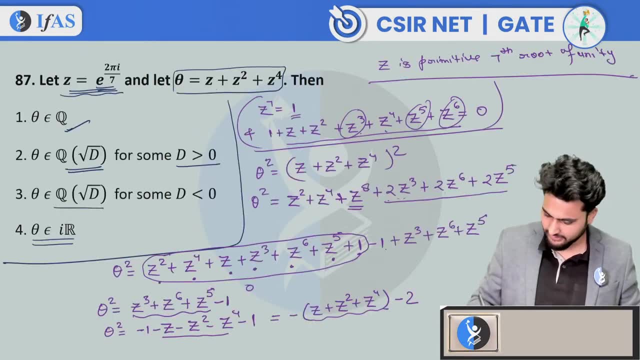 So what equation did we get in theta? What equation did we get in theta? Let's see. We will have to take some time to understand this. If you are in a hurry then you won't understand. theta square equals to minus theta. Is this theta? 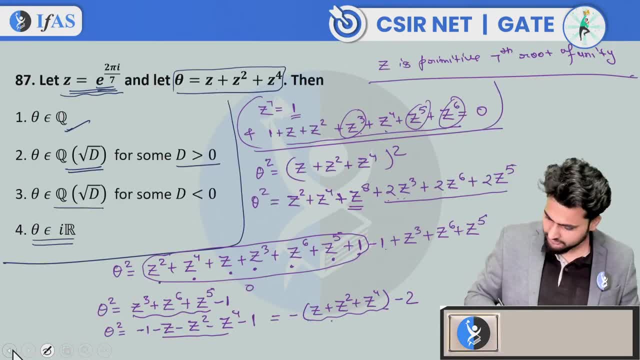 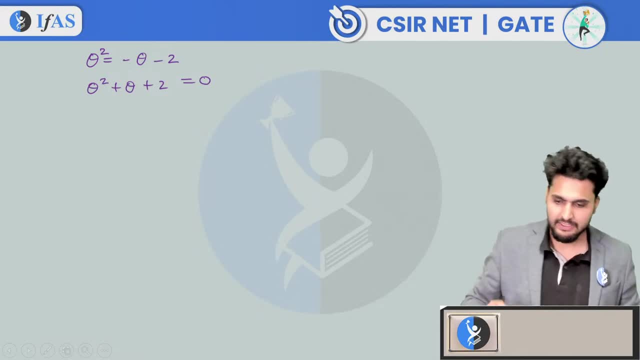 minus theta minus 2.. minus theta minus 2, or plus 2? minus 2.. So we got an equation in theta: theta square plus theta plus 2 equals to theta. From here I will write the value of theta: theta is equal to. 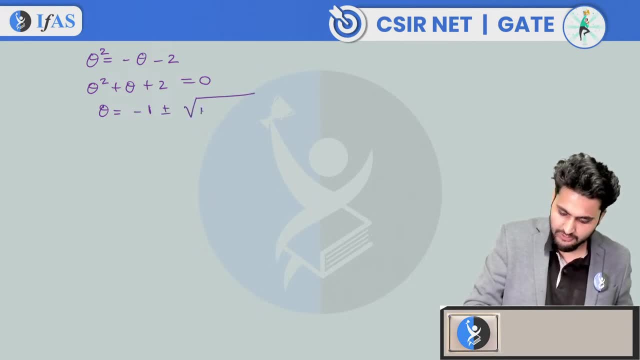 minus 1 plus minus square root of b square, which is 1 minus 4ac, means 8 upon 2k, So this is 2.. So this is minus 1 plus minus square root of minus 7 upon 2.. Can you say anything now? 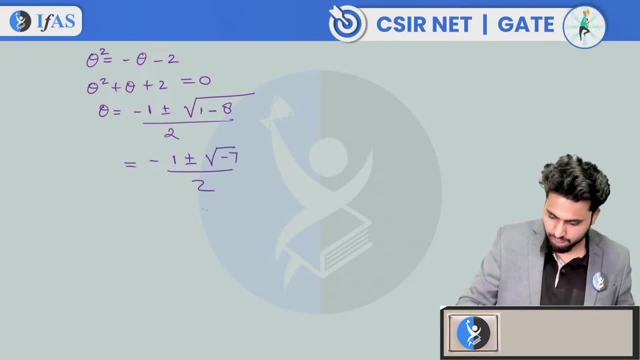 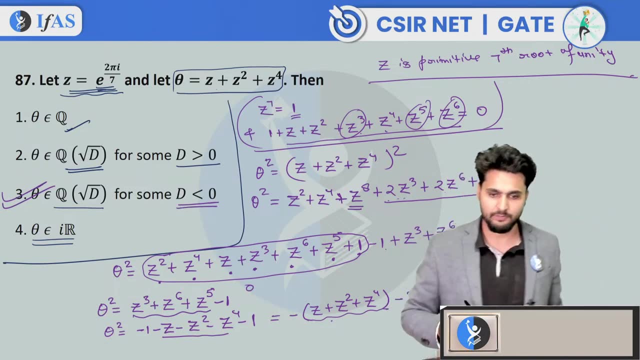 minus 1 plus minus. That's it. What can we say now? Where does theta belong? theta belongs here For d less than g. So c is the correct option, d is the correct option. Is that clear to everyone? Why? 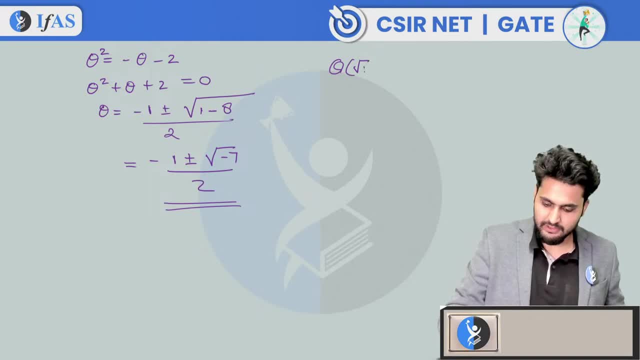 Because when you define q square root of d, then how do you define it? q square root of d defines as a plus b square root of d, where a comma b belongs to q. But if you look at it from here, where does it belong? 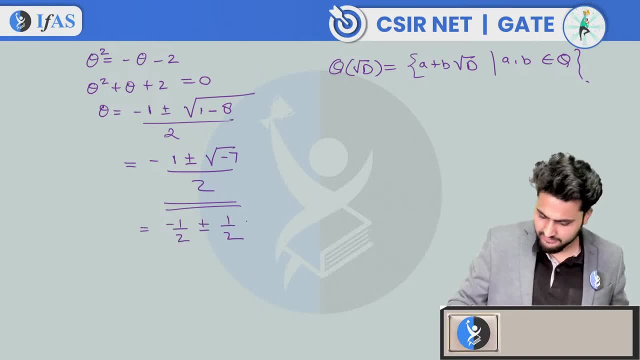 If I write it like this: minus 1 by 2 and plus minus, let me say 1 by 2, square root of minus 7.. Can we say that this belongs to q, square root of minus 7?? q, square root of minus 7.. 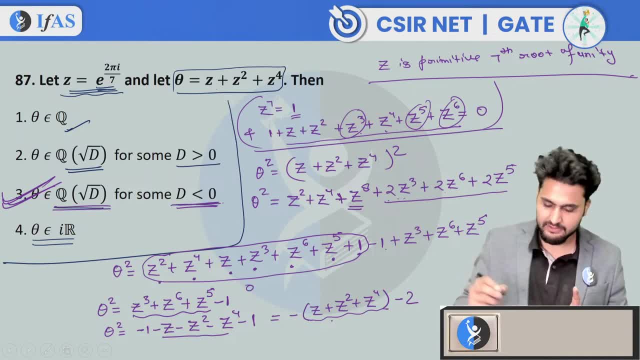 What happened to this? q? square root of minus 7 is also at least less than 0.. Those who were saying: are you clear now Or are you confused? We will do one more question After dense. we will stop here for today. 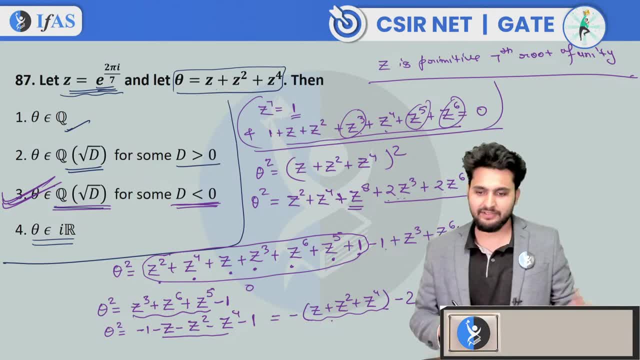 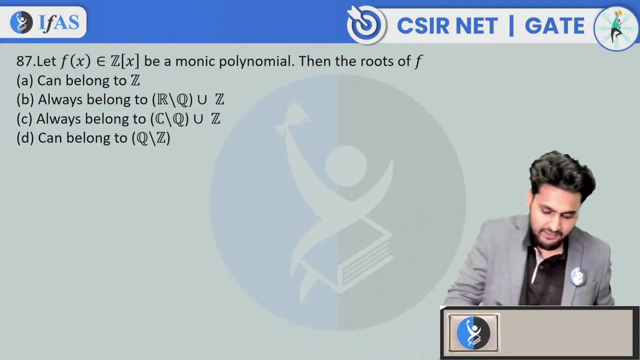 In the next lecture we will discuss further linear labor or linear theory. Try one more question. This is also a good question. Let f of x belongs to zx. f of x is a member of zx. This is also a very good question. 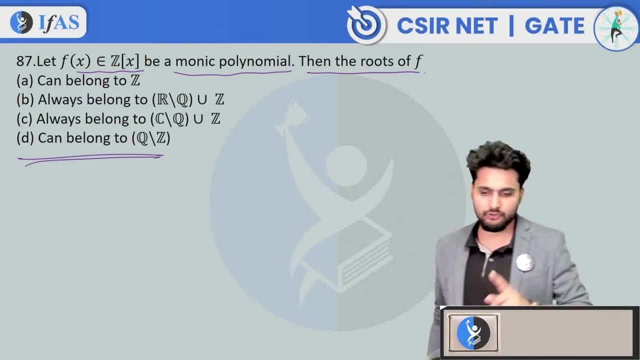 Then the root of f? Where will it be? Think about it: If f of x is a monic polynomial of zx, then where will the roots of f be? Can it belong to z? Can it be in z? Always belongs to r minus q union z. 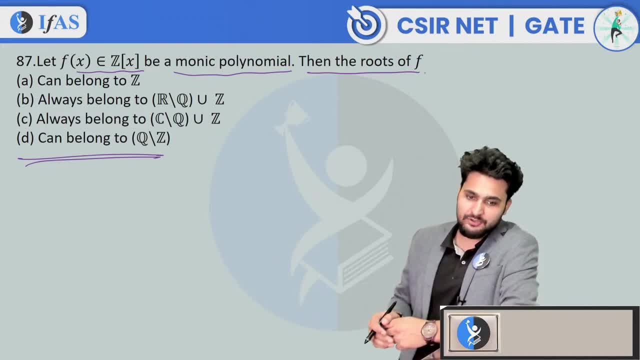 Always belongs to r minus q union z. Always belongs to c minus q union z. Always belongs to c minus q union z. Or can it not be in q minus z? Can it belong to q minus z? Then it belongs to q minus z. 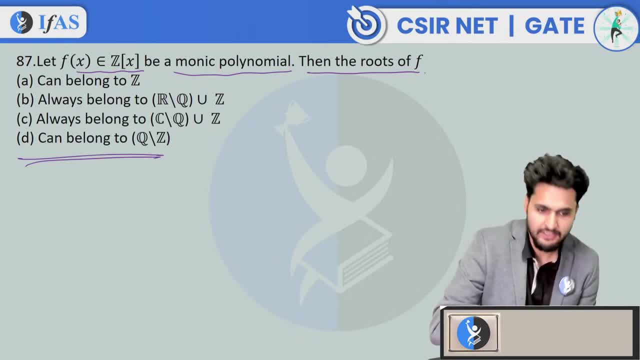 What do you think These are good questions. These are the previous questions of CSI. It may take some time, but you should think about it. If you think about it, many things are used to make simple questions very easily. Think about such questions. 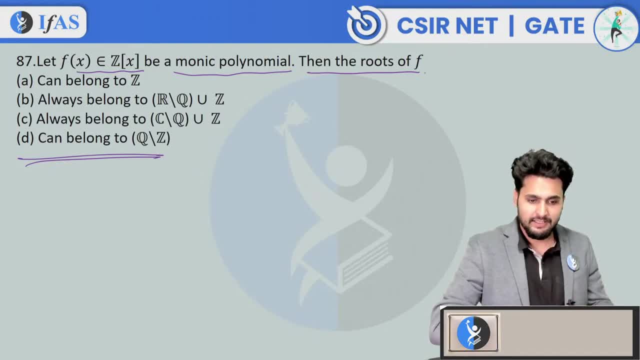 Many such results will be used. If you know the results, then you can make many simple questions very easily. Think about it. If you know the answer, we will see that c is correct or not. you are right. c is the correct option. 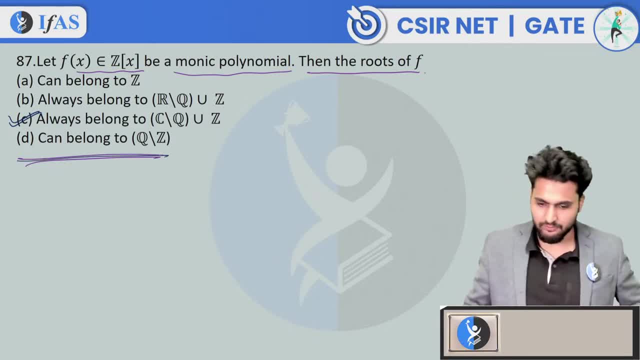 See, do people think c is correct or not? I will explain how c is correct Or I will leave it for you. Think about it. I have told you that c is correct. If you want to know the correct answer, then please comment. 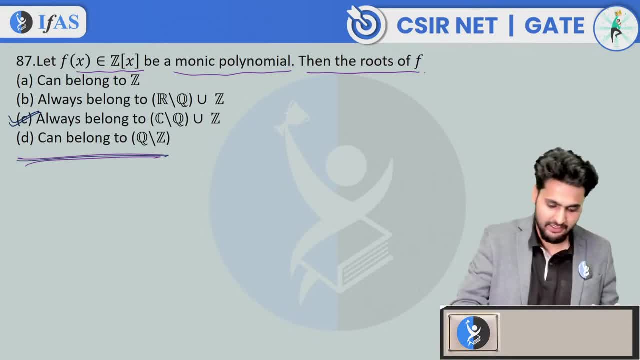 and tell me why c is correct. one is also considered it belongs to z. this is also correct. you can consider: let me say: x square minus one equals to zero. this is a modic polynomial. what is a modic polynomial? 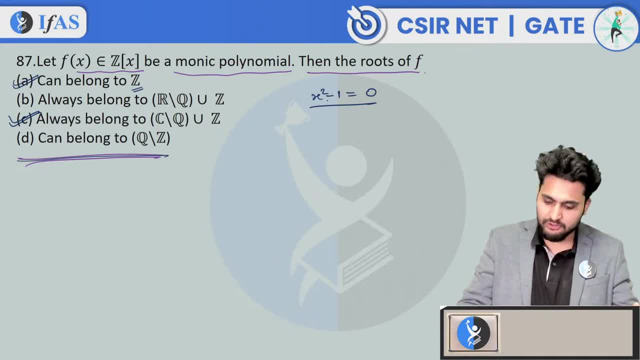 its leading coefficient is one. its leading coefficient is one: it has zx polynomial. its roots are x, equals to plus minus one. they are belonging to z. this is also correct. so a and c, both are correct. if you want to know the explanation of this, 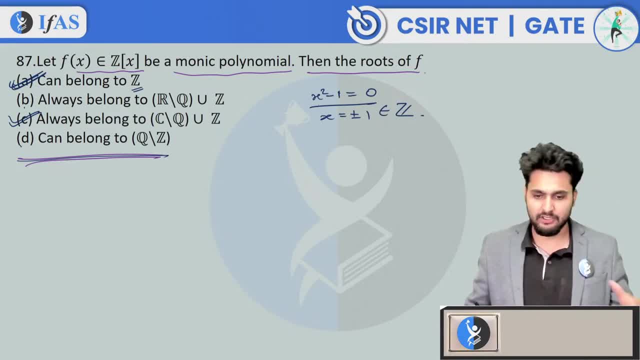 and why b and d are wrong and why a and c are correct. if you comment and tell me, we will talk about it in the next lecture. otherwise, if you are satisfied with the answers of the questions, then no problem. this is all about today's lecture. we will stop here for today. 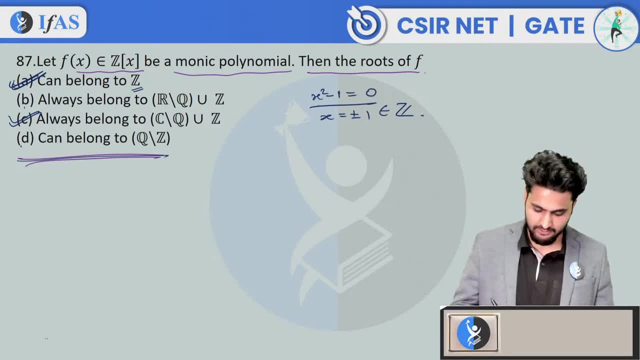 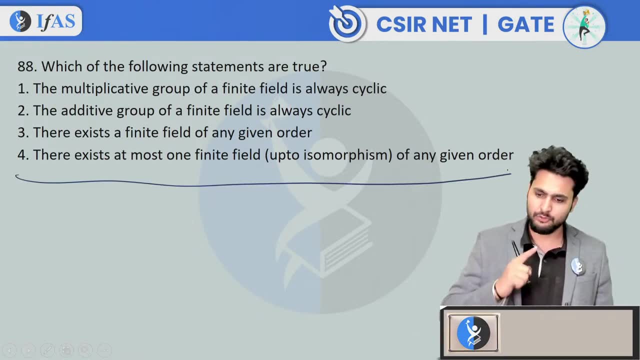 thank you very much for joining and we will meet in the next lecture. take care of yourself. if you want to do one more question, I will not give you this question in the homework. you can answer it in the comments. think well before answering. just don't waste your time. 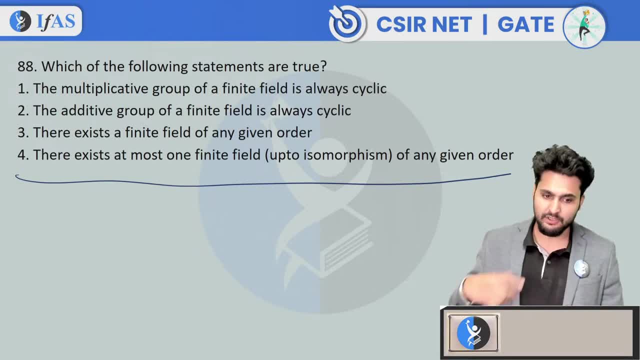 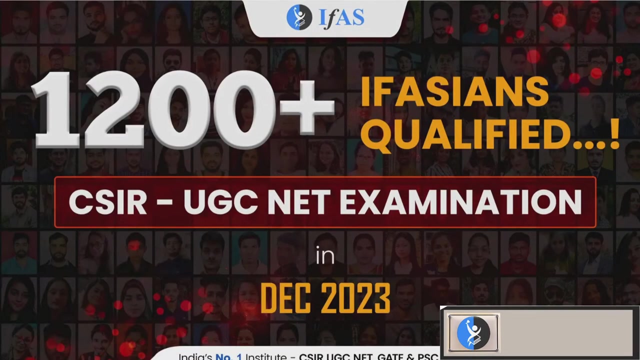 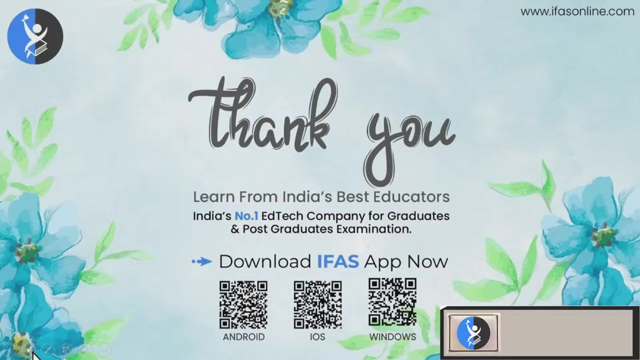 count the examples, say: cancel out, take care everyone, and we will meet in the next lecture. thank you very much, Thank you, Thank you.